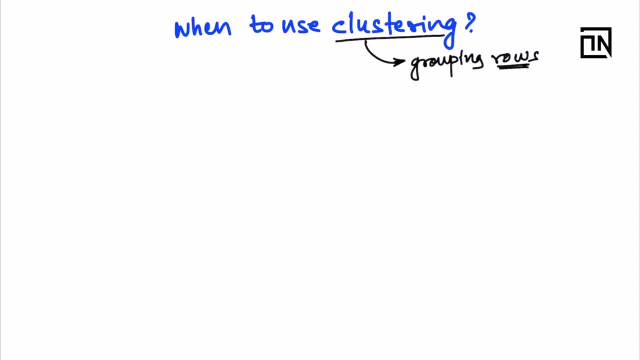 in data. So the very general idea about cluster. if I had to summarize it in one diagram, I can build this. So let's say you have some data set and it has multiple rows and you would want to understand, let's say, row number 1, 2, 3, 4. there are thousand rows, so you would want to understand whether row 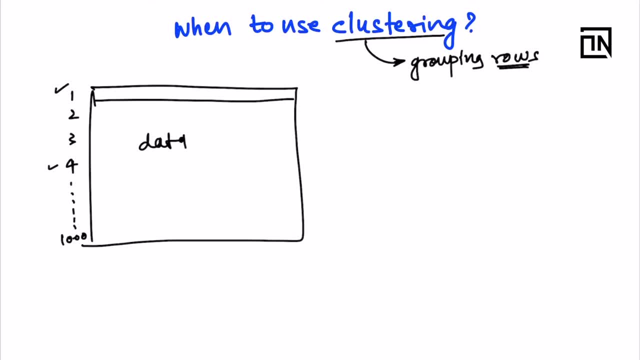 number 1 is similar to row number 4 of data, or row number 3 is similar to row number thousand, or row number 2, 3, 4 and thousand. all these are similar and they belong to one particular group. so, using clustering techniques, using clustering, what i can do- there will be multiple columns. 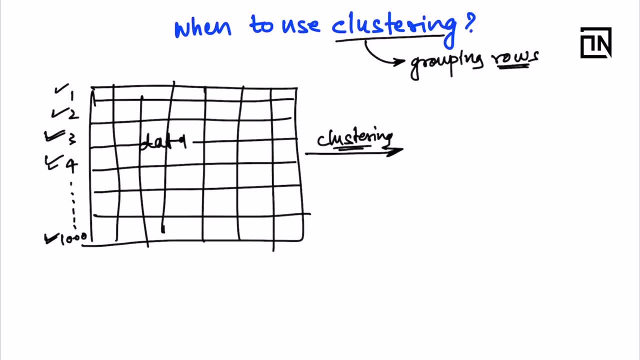 obviously it's a tabular data, so there are multiple columns and based on these columns i'll try to group them together and i'll try to find out that in this data so and so rows are similar. let's say row number 1, row number 10, row number 11. 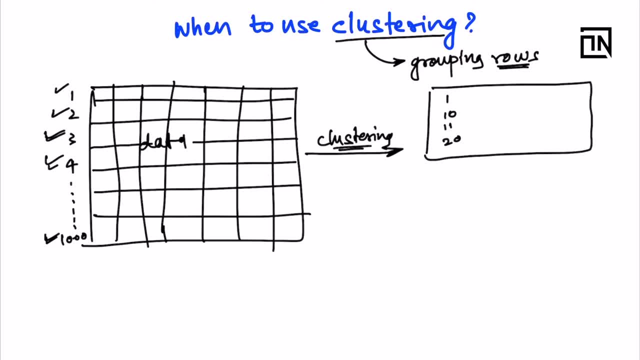 row number 20. these are similar, so on and so forth. then there are a couple of other rows which are similar, and then there are couple of other rows which are similar. and just for the sake of explanation, let's say there are thousand rows. so 600 rows came over here and 300 rows came. 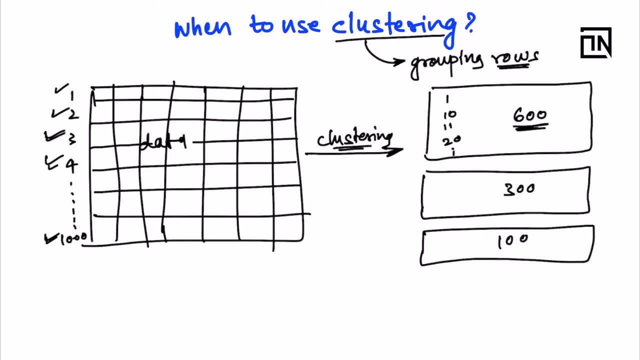 over here and hundred rows came over here. so the idea of clustering is to find out what, What kind of rows in the data, what kind of data points which I have. they are similar. So the key idea of clustering is to find out which rows can be grouped together. 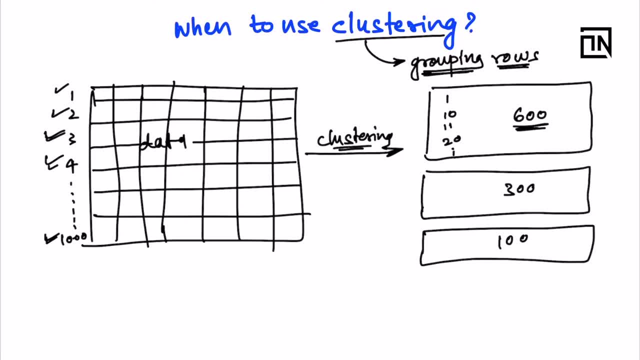 So it is used to group the rows, and why would I do that? So this will help me to take certain action on this group of data and some other action on this group of data and some other action on this group of data. So, to consider a simple example, let's say online shopping. 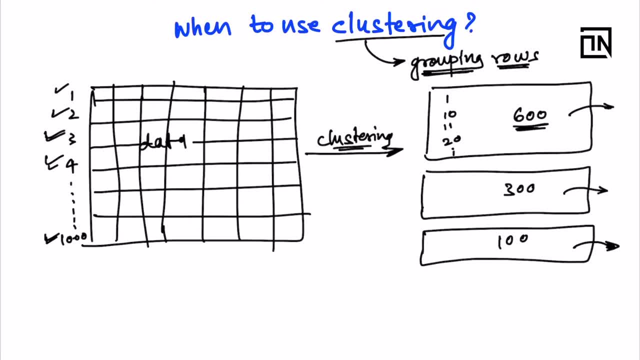 So you have the online shopping data with you, And this online shopping data set contains different scrolling information about all the users like which product they are eyeing, which product they scrolled, which product they did not like, how many seconds, how many seconds did they stop there and how many times. 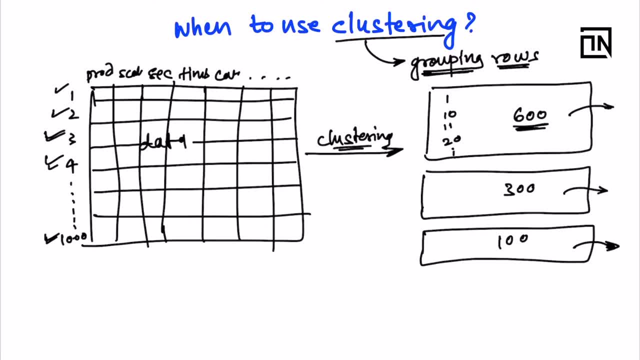 they came over there, what is the category of the product, so on and so forth. there will be a Huge amount of data which is captured the moment you scroll through any product on Google, let's say, or on amazoncom or flipkartcom, any, any shopping website you scroll through. 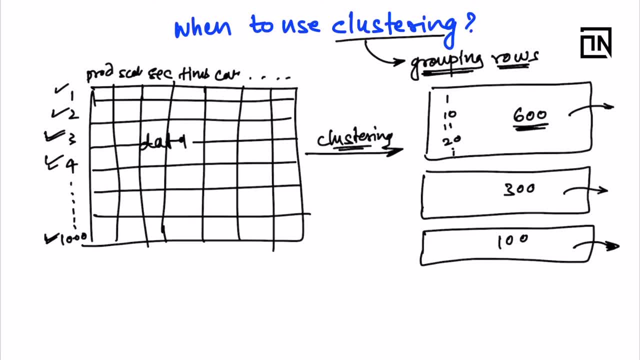 any product and that data will be captured by these companies to analyze and to give you better recommendations for products or better suggestions for products. What clustering helps us perform in this scenario Is it will group all sorts of similar behavior, like all the people who are interested in. 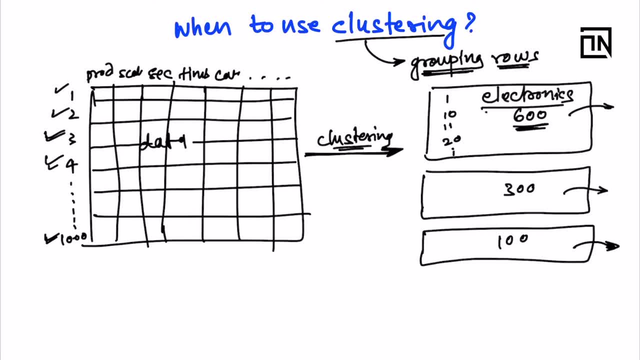 let's say, electronics. So they are interested in the MacBook, or they are interested in some Samsung phone and they have been eyeballing these kinds of products. So all those rows, all those consumers, will be grouped in one particular group. Then some other people might be interested in, let's say, books. actually I should keep. 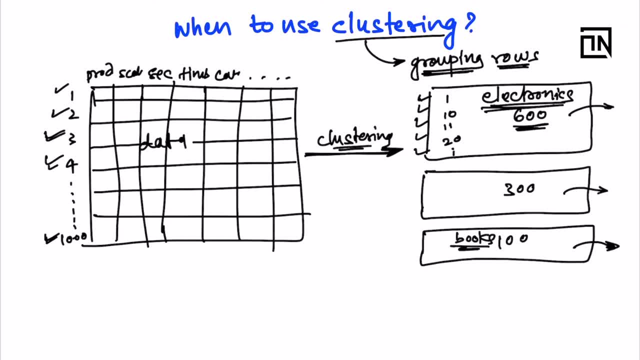 this books. here, Less people are interested in books. So let's say, some people are interested in books and some people are interested in apparel. So, if I am able to find out- okay, these are the customers who are interested in apparel and these are the customers who are interested in books- I'll be able to take certain actions. 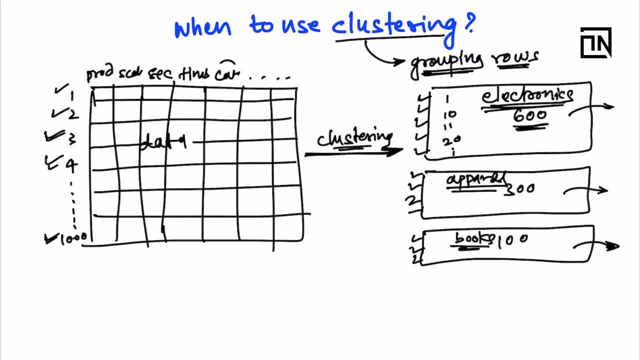 Now you will say: why can't I simply do it based on the category of the products, So you will miss out on certain opportunities, like the person might be interested in electronics plus books, So that is one group or apparel plus books, or books plus electronics. 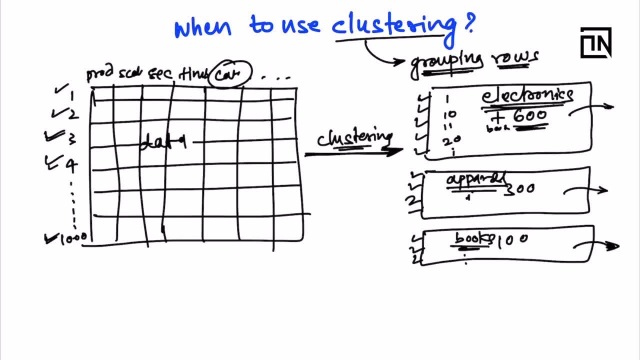 So there might be certain behavior of the consumer which you may not be able to select or bifurcate just based on the category of products. So what you need to do is to take help of clustering and, based on all the data points which has been collected for that user, which particular row is similar to row number. 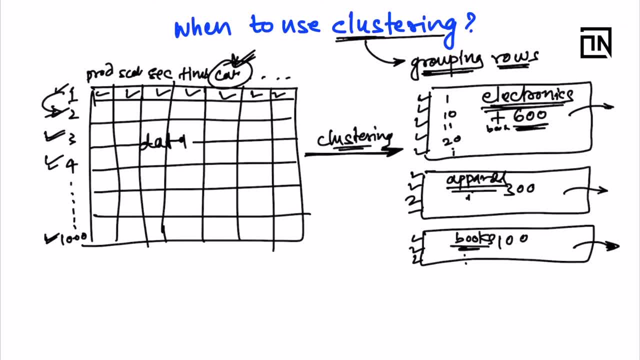 Let's say, one will be grouped with row number one. So whether second row is similar, third row is similar, fourth row is similar, all of this comparison will be drawn and whichever is similar will be put under one group. And once you have this group, you can start taking some actions specific for that group. 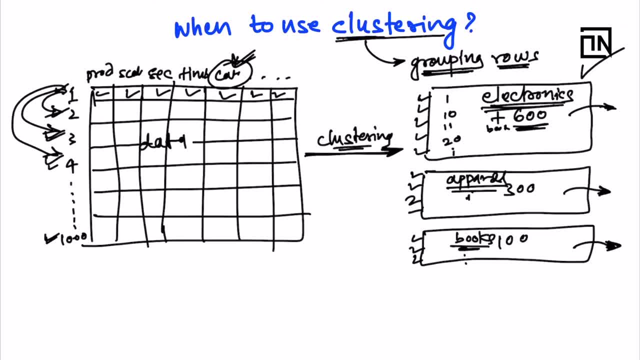 Because, let's say, if you want to promote the sales of books, so you cannot give the coupon to each and every one in the customer base. You have to focus and target only for people Who are interested in books, otherwise your campaign will have a lot of unnecessary noise. 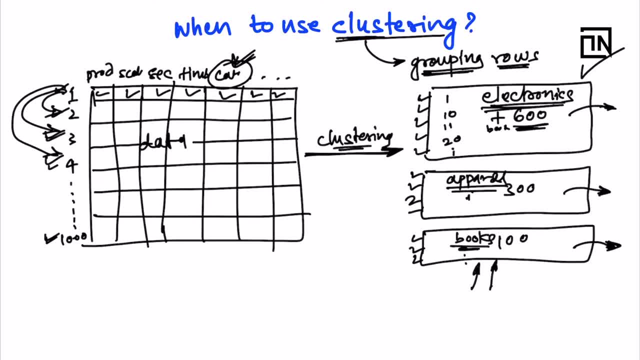 because you will not be able to sell through those coupons to other people who are interested in electronics or apparel. They are not interested in books. So this is the main idea behind clustering: We want to group the rows, group similar rows and then take certain actions on it. 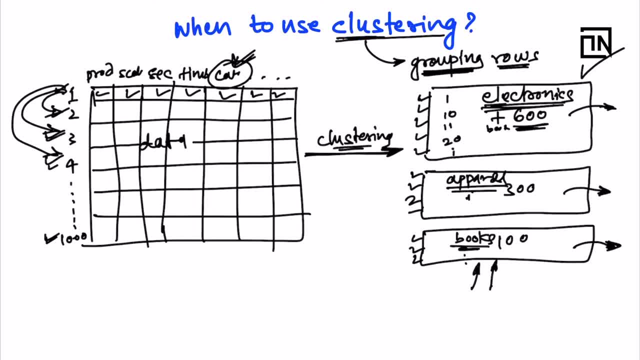 Now, this is a very general idea. This can be applied to all sorts of industries. Another very good example In which I also have experience in is telecom. So whenever you make a call, there is a CDR generated, a call detailed record. 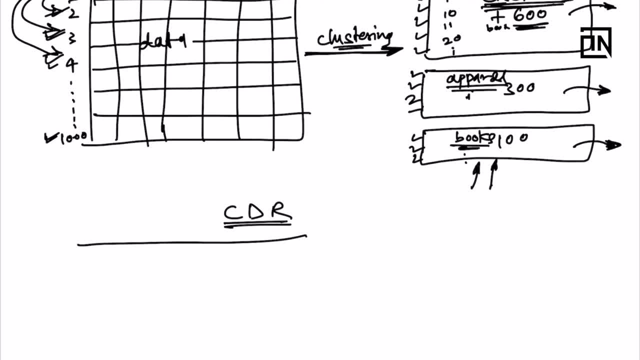 And based on this CDR, I can literally understand the behavior of my customer, like: from where the call originated to where the call went, how many number of minutes the call was on Then? how was the network type? Did the call drop? 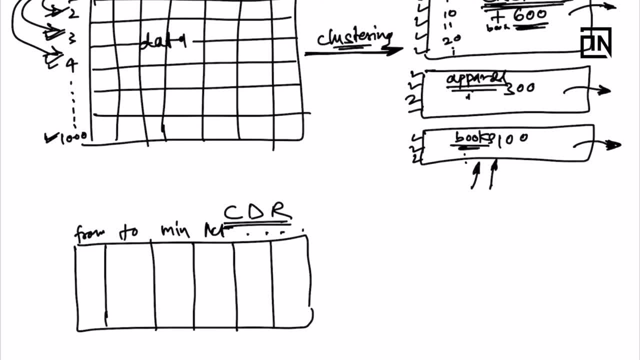 And once again called: How many minutes, So on and so forth. So there are so many data points which are collected in the CDR And based on this, you can group the customers, the type of customers, and then take actions. 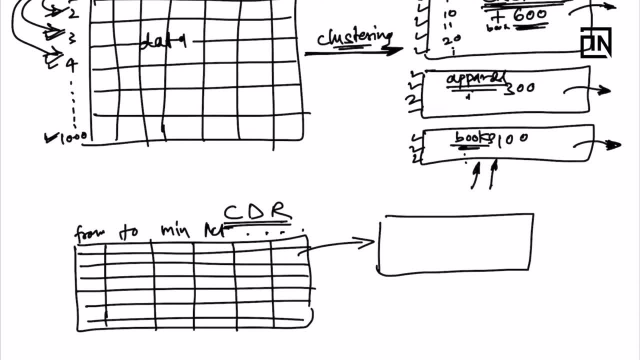 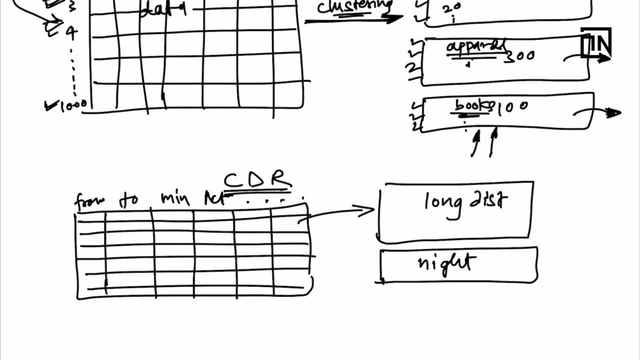 on these type of customers. So let's say you get one group who is long distance calling people. You get one group who are calling majority of the times in the night, probably young college students, And they're chatting a video And they're chatting up with their friends. 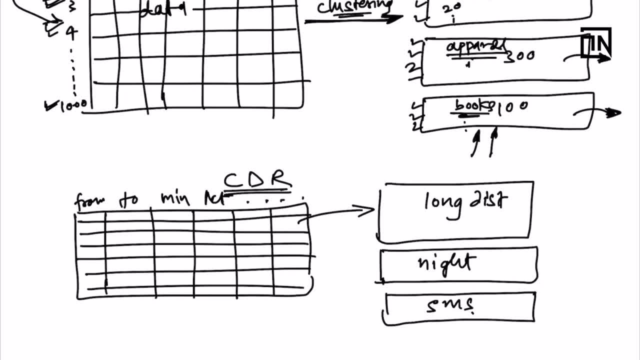 And some other people who are mainly communicating with SMS, So on and so forth. So there are different kinds of patterns which may come up, like long distance plus SMS, or night plus something else. So different behavior which cannot be grouped by just one particular column. 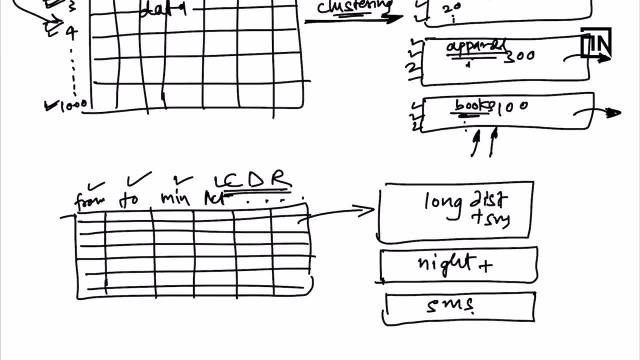 So you need all the columns, information, And then, based on that, you try to see this whole row is similar to which row, this row, or this row, or this row, and then group it. Now, here I'm drawing three, three groups. 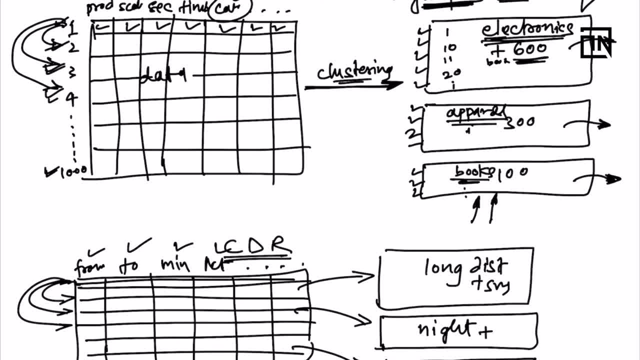 So how many number of groups are possible? So that is up to us- And going further, I'll discuss it- that you can provide the number of groups and clustering algorithms like k-means, hierarchical clustering and db-scan and optics. 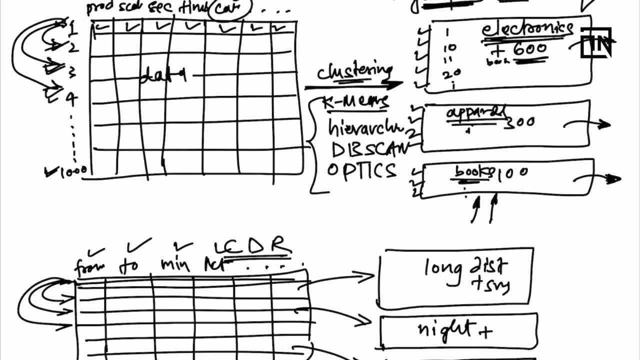 So all these algorithms are nothing but clustering algorithms. they work slightly different from each other, So if you pass this data to k-means, it will give you certain groups. Now this behavior which you got here is known as unsupervised. 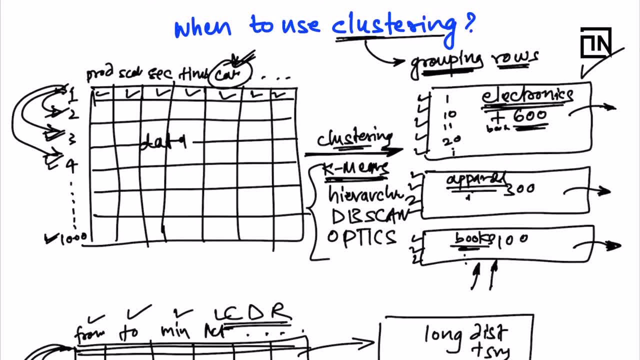 Why it is unsupervised. During this whole discussion did I mention any time about a target variable like? did I train my clustering algorithm that when you see these kinds of data inputs then tag it to group number one or tag it to group number two? 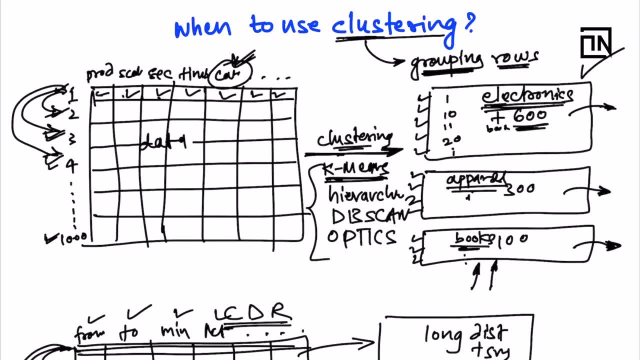 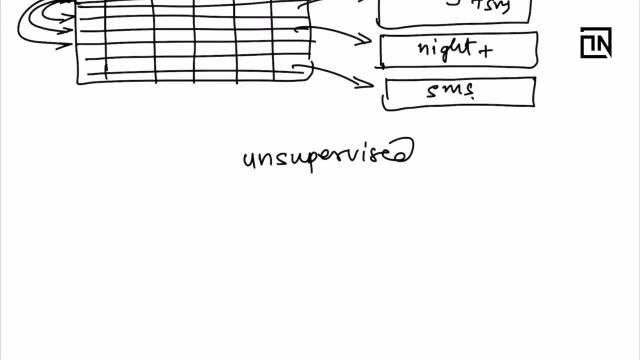 We did not. That will become classification. So in clustering the real hallmark is it is unsupervised. So when it is unsupervised there is no target variable. That means if I have a data, I don't know much about it. I just have these columns. 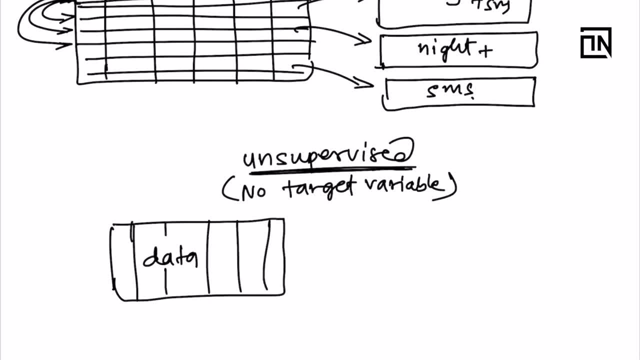 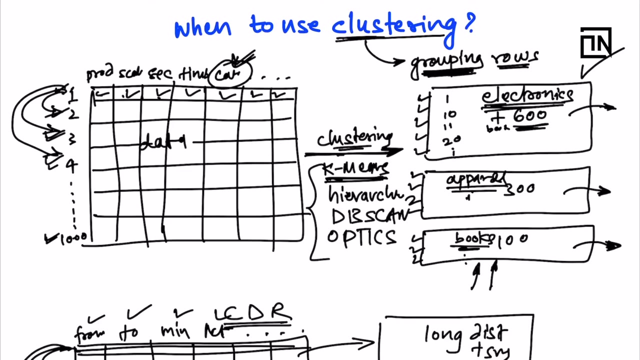 I can pass this data to the clustering algorithm and it will give me certain groups from it. So this whole operation is unsupervised. Okay, because I just pass the data and get some results. So why do we use clustering? We use clustering to group similar rows and then take action on all those similar rows. 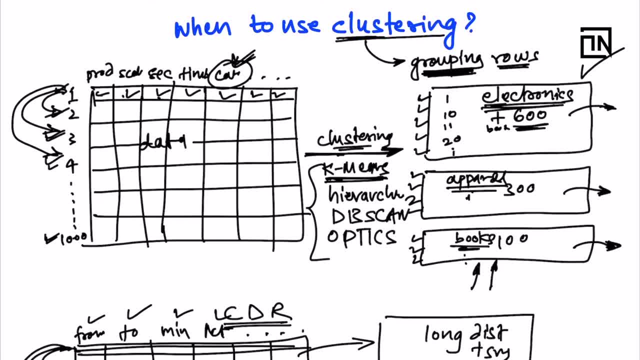 and maximize our sell through or maximize our results. Now, how do I find whether this row is similar to row number two or row number two is similar to row number three? How do I find this? So, to understand this concept, let me take you back to your class seventh, where you did: 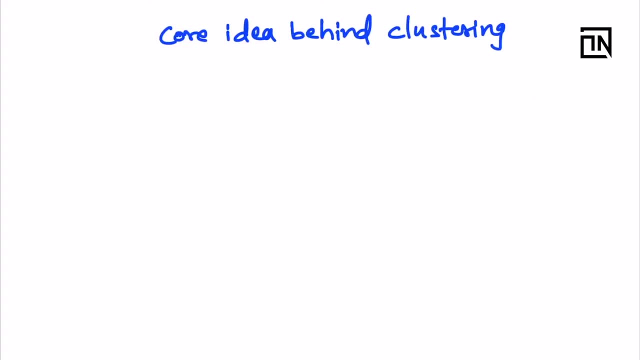 some kind of simple plots at the back of your notebook in the green colored graph charts, and that describes the core idea behind clustering At that time in 7th standard. we never knew that it will come back to us and we'll be using it again. 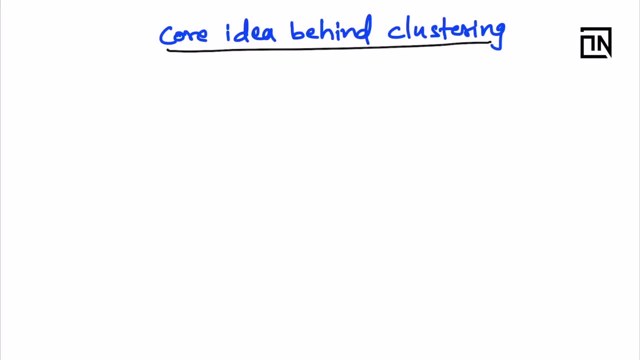 But here we are. So the core idea behind clustering is Calculus. Calculus is a function of calculating distances. Distances means what? So consider this example. So you have x axis and y axis, and in our 7th standard we used to plot certain points. 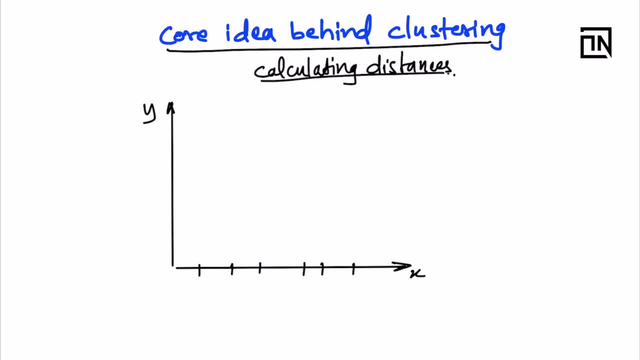 So you can count 1,, 2,, 3,, 4,, 5,, 6,: 1,, 2,, 3,, 4, 5.. Okay, So let me plot the first point, which is 2, 4.. 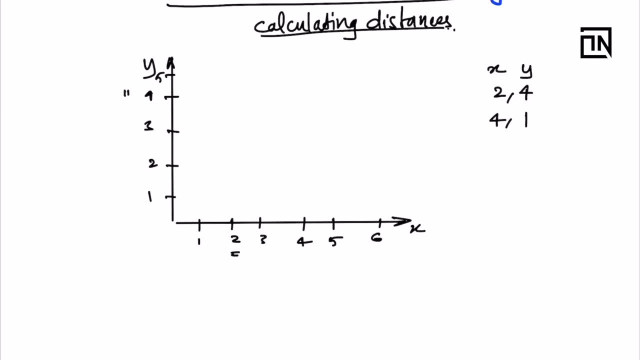 So 2 in the x axis and 4 in the y axis. So it will be plotted somewhere around here like this: Let me call this point number A, So this is A. Similarly, 4, 1 will be plotted somewhere. 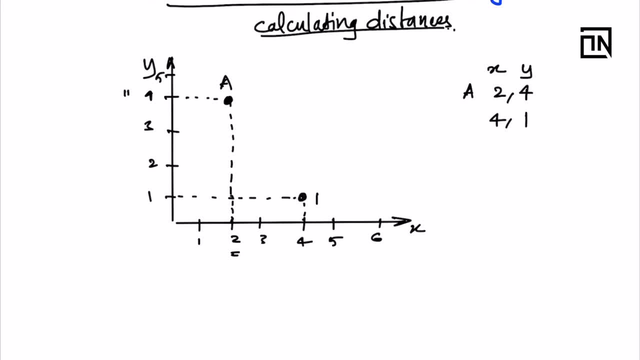 over here. Let me call this point B. Now let me plot one more point C, and it is plotted at 6, 2.. Okay, So 6 in the x-axis, 2 in the y-axis, somewhere over here. C Now visually, if I ask you which? 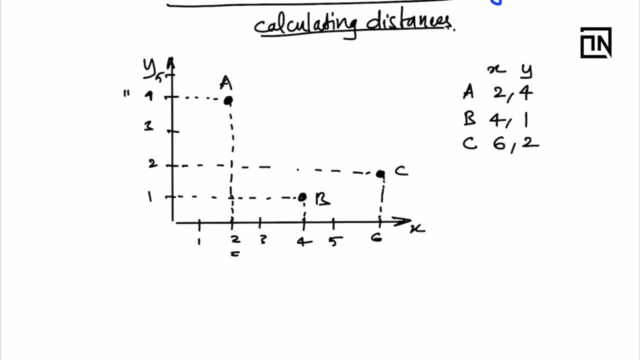 point is closer to B, So you will say the point C is closer to B. Why? Because you can see the distance is smaller. This distance is smaller than this distance. It's very easy to visualize. Now how do we calculate this distance? So distance can be calculated between: 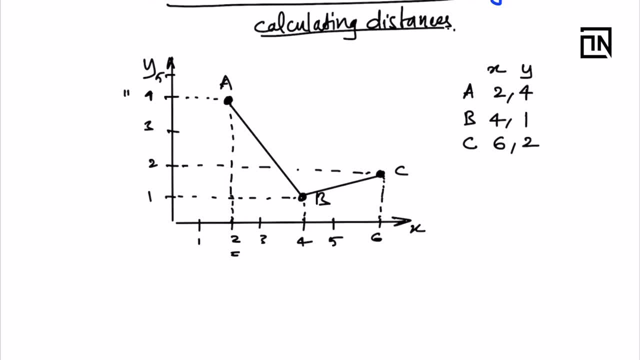 two points using the Euclidean formula, by subtracting the coordinates, So distance can be computed as x1-x2, whole square between two points, plus y1-y2 whole square, so on, so forth. Under root of that, So for example, let's say, distance of A and B can be calculated as A and B, So 2 is the. 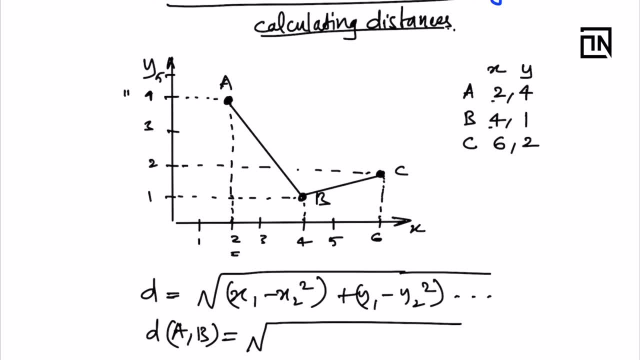 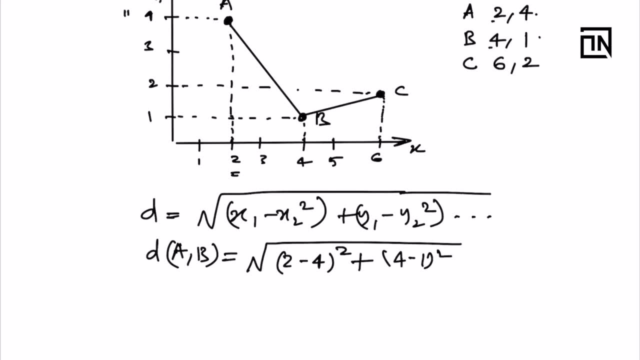 x-axis of A and 4 is the x-axis of B. So I will say 2-4 whole square plus 4-1 whole square. Similarly, if I have to calculate the distance between B and C, I will say 4-6 whole square. 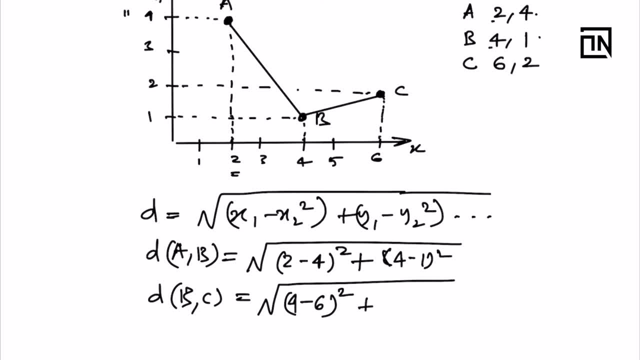 plus 4-6 whole square plus 1-2 whole square. So whether I do 4-6 or 6-4, it doesn't make any difference because it is going to be squared and added. So if you really calculate this distance and this distance, you will. you will find. 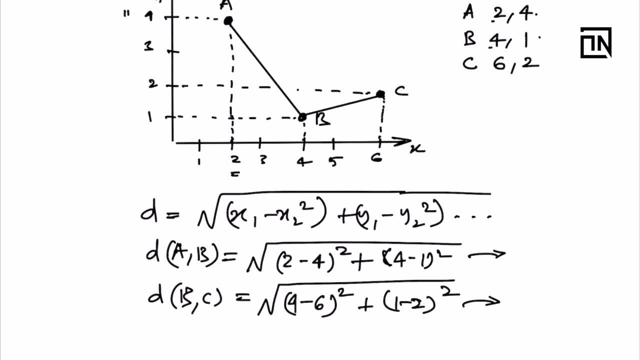 out that the distance between B and C will come out to be a smaller number and distance between A and B come out comes out to be a larger number as compared to each other, And you can see that in the diagram also. So this 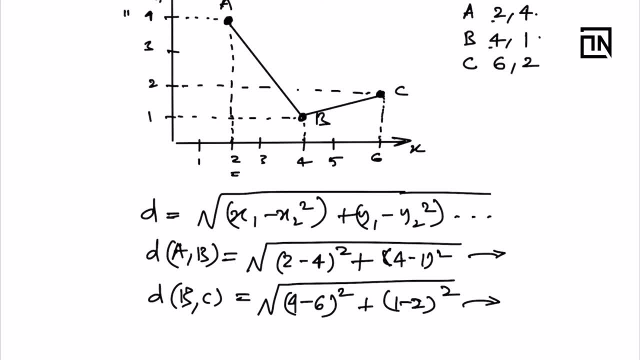 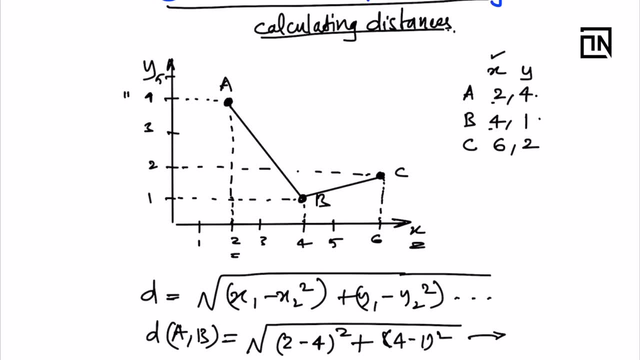 this expression gives us the distance between two points and these two points right now are in two dimensions, so dimension x and dimension y. so you can imagine this column and this column being plotted over here. these are two columns in the data. if i add one more column, let's say z, 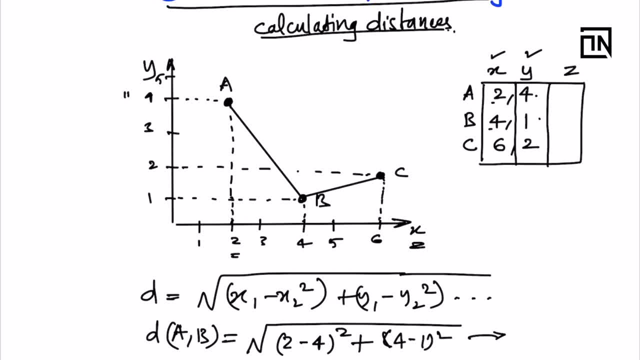 column. so the point is now being plotted in the three dimensions. so i'll extend this diagram in the 3d and then i'll have to point. then i'll have to plot these points in the three dimensions. so let's say two comma, four comma, three four comma, one comma, two, six comma. 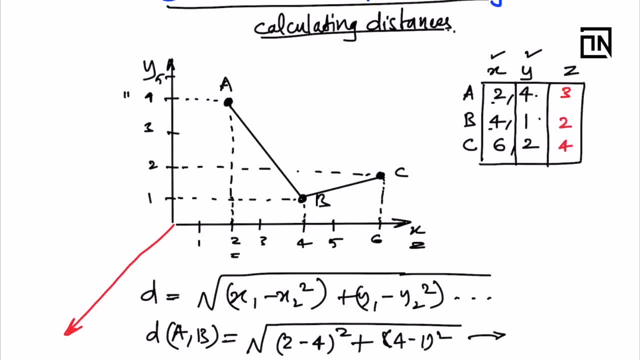 two comma four, just some random numbers so you can count all these points in the z axis. so one, two, three, four, five and then a will be somewhere. the point a will be somewhere over here and B will be somewhere over, so I'm not drawing it, because it will. 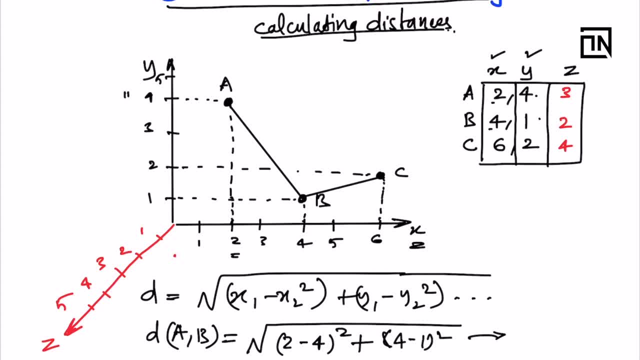 mess it up, but you can imagine that it will come. it will come into the three dimensions now because there are three columns now in the data. if there are four columns in the data, then there will be four dimensions and five dimensions. but you can imagine this. a is nothing but one particular point. B is also one. 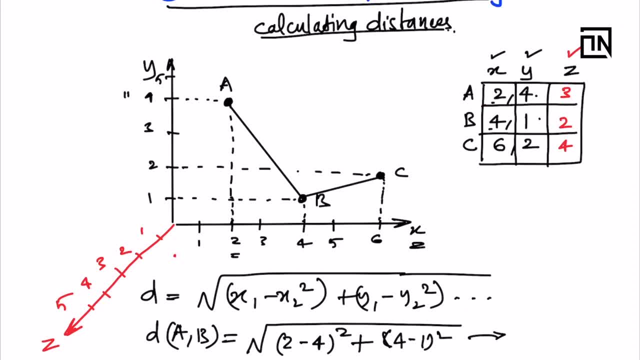 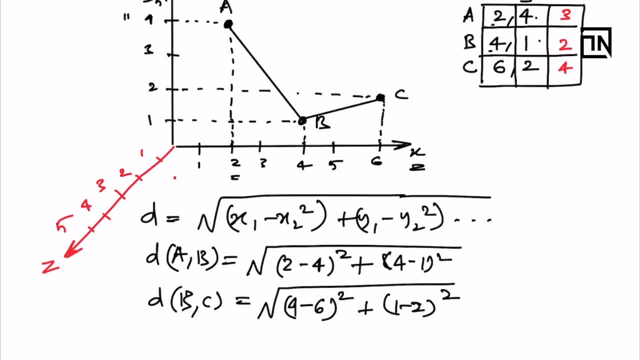 particular point and C is also one particular point. so now, if I have to calculate the distance between a and B, how do I calculate? I'll simply extend this formula and say 3 minus 2 whole square, and once again, between B and C plus 2 minus 4 whole square. so if there are more columns or more dimensions, I'll 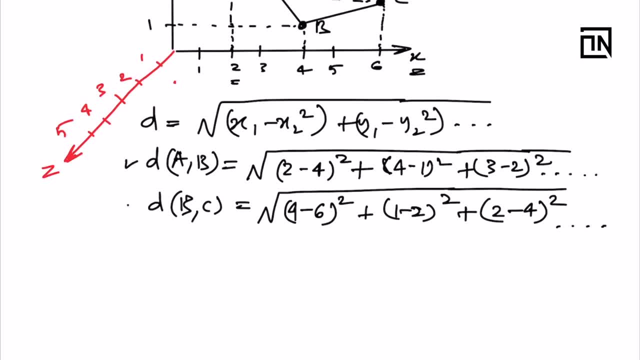 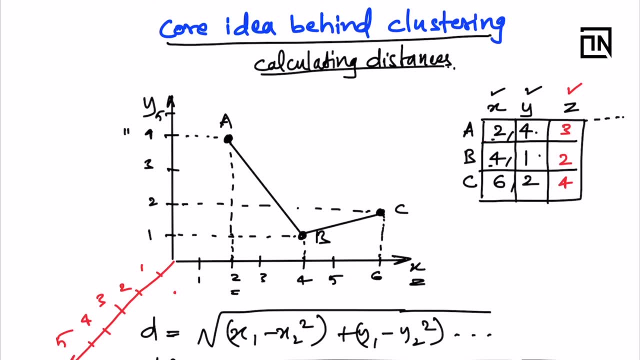 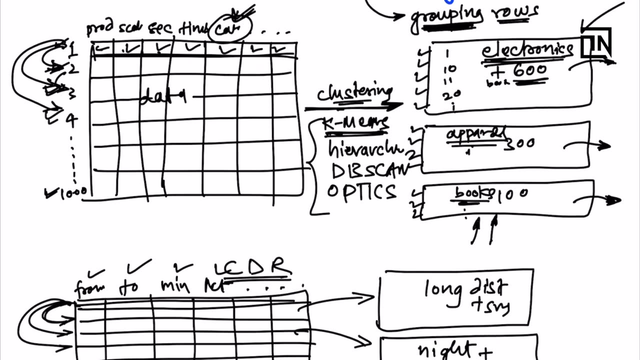 simply keep extending this formula, okay, and I'll get the distance you. and this exact thing happens in my clustering algorithm also. so the whole clustering algorithm is based out of this principle: that when you are saying that this row is similar to another row, so what you try to do is you try to subtract the distances or subtract the values of the first row. 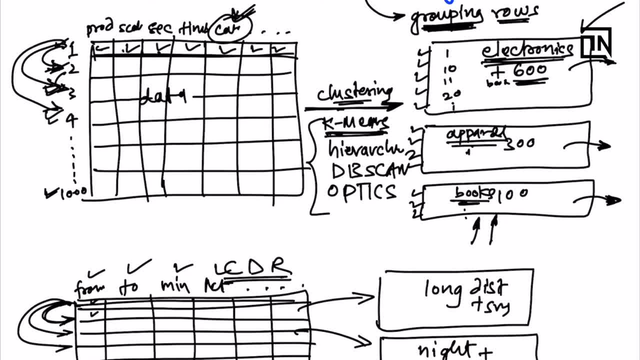 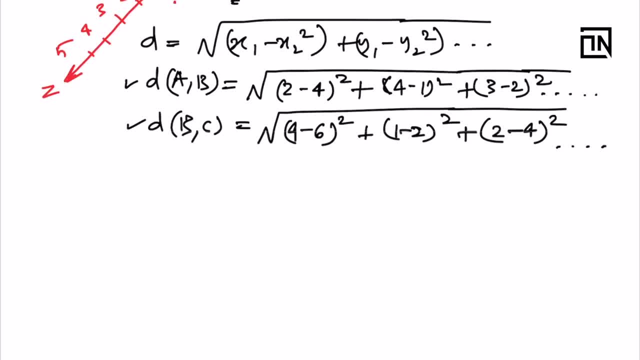 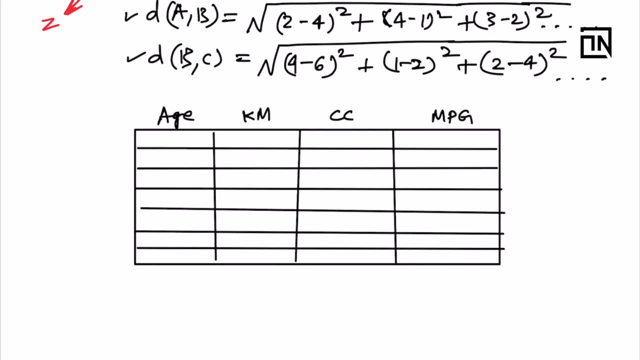 and the second row, and then look into the distance in those many number of dimensions equal to the number of columns and then decide whether it is really similar to this or not. so just to give you an example, let's say you are, you are having a data set like this. so let us say you have this data. 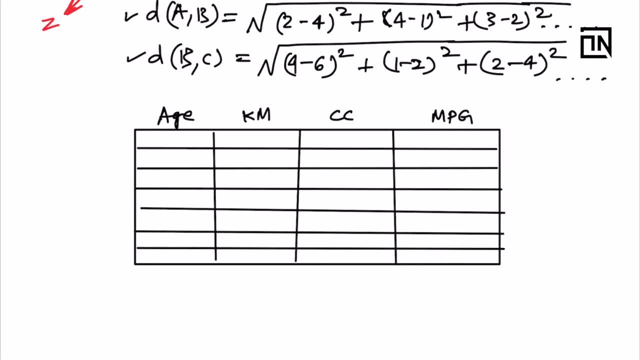 which contains the age information of car in months, the number of kilometers it has been run, the cc of the engine and the miles per gallon, and you would want to use this data to understand what kind of cars do you have and group this data accordingly. accordingly. now, let's say, let me write some dummy numbers to help you understand. 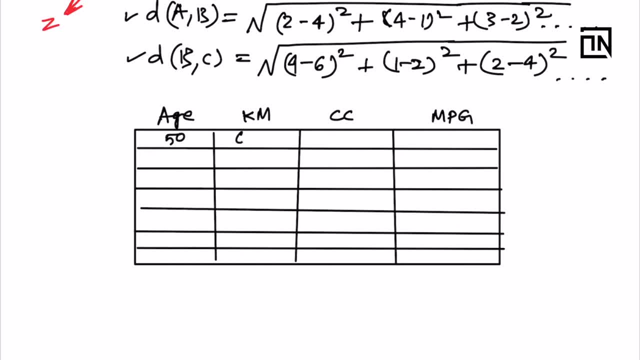 let's say, age is 50 months, the number of kilometers is 60 000, cc is 1200 and miles per gallon is, let's say, 35. another car is there which is 55, 67, 000, 12, 50, 30.. another car is there, let's say 10. 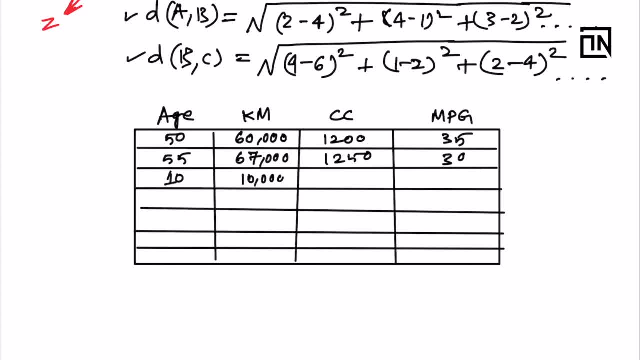 10 months and it has been run for 10 000 cc is 1100, miles per gallon is 35. so if i just take these three examples, let me call this car number a, car number b, car number c. so car number a is similar to car b. i can see the values are quite similar and car number. 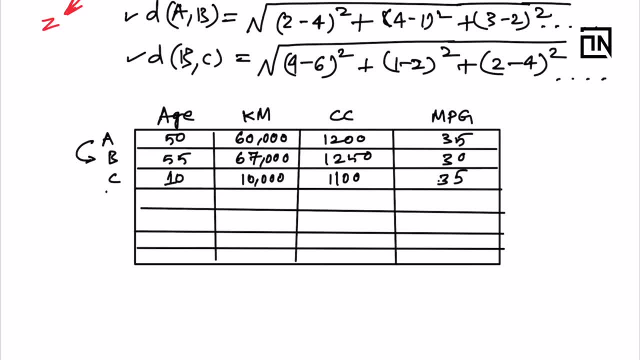 two is similar to car b and car number c is not similar to a and b, both okay. so if i have to figure out whether a is similar to b or a is similar to c, by looking at these values, i realize that, yes, a and b are looking quite similar because the numbers look similar. now, if the numbers are, 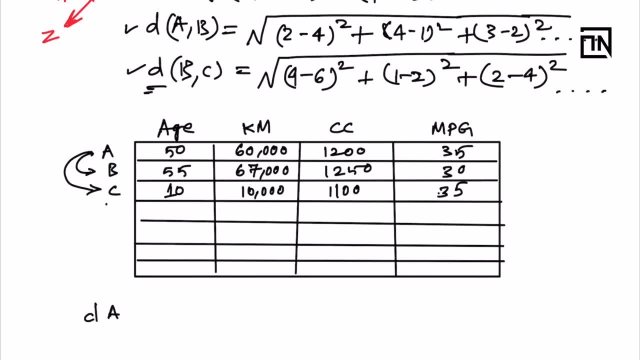 similar, then what is going to happen in this formula? if you calculate the distance between car a and b, how will you do it? so you will use age dimension subtracting the values first, like 50 minus 55 whole square, plus the kilometer dimension: 60,000 minus 67,000 whole square, plus 1200 minus 1250 whole square. 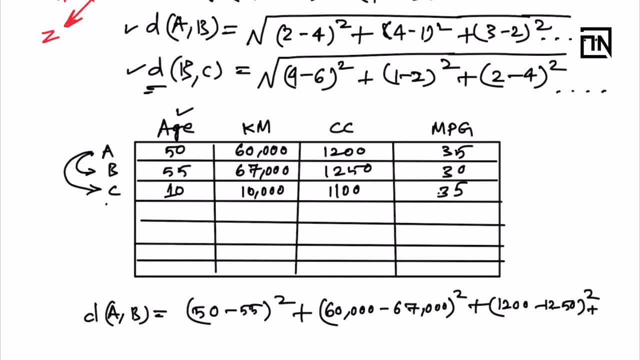 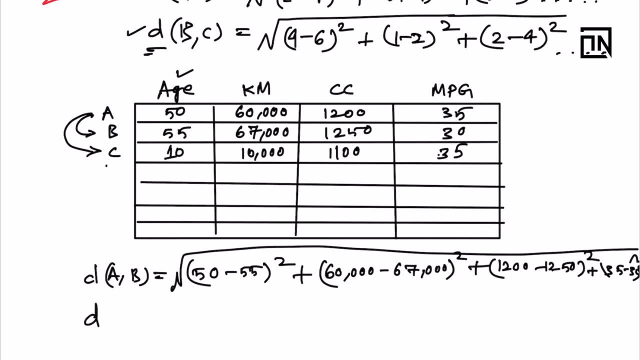 so on, so forth: 30- let me write the last one also- plus 35 minus 30 whole square and take the under root of this. now, if you calculate the distance between a and C, okay, so 50 minus 10 whole square plus 60,000 minus 10,000 whole square, plus. 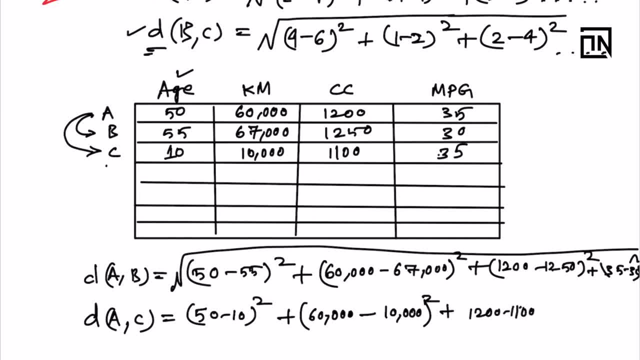 1200 minus 1100 whole square, plus 35 minus 35 whole square. so you can literally see there are certain figures which will generate huge amount, like this: 50 minus 10 and 60,000 minus 10,000. this is going to generate huge number and due. 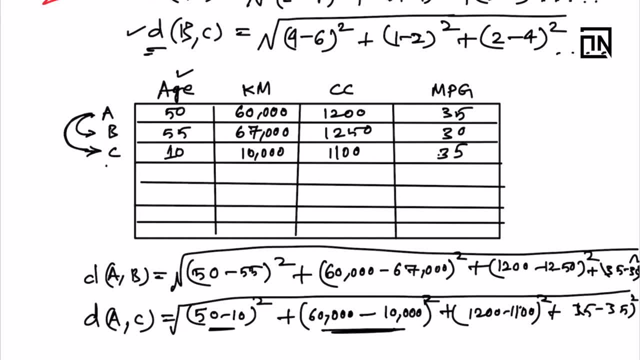 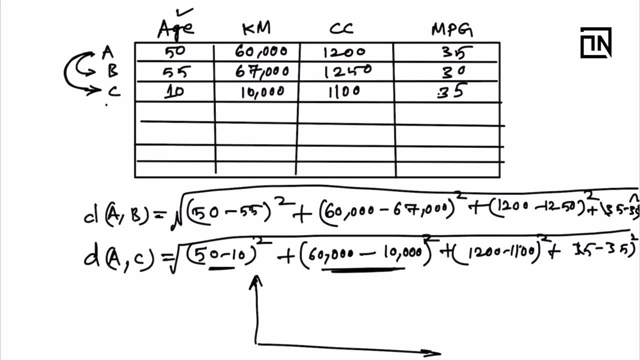 to that, the distance between A and C is going to come large. so if you try to plot this data and try to see in three dimensions- or sorry, one, two, three, four dimensions, I'm just plotting two dimensions. point number A will be somewhere, let's say, around here, and point number B will. 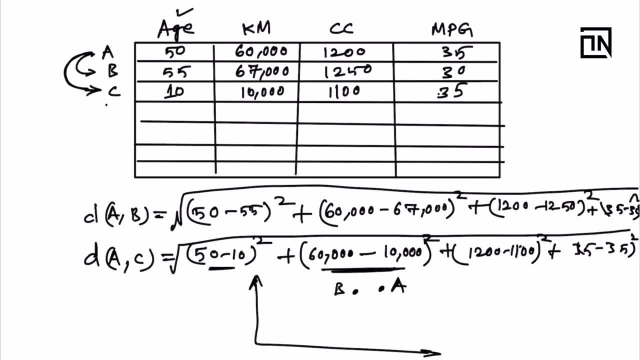 be somewhere close to it. point number C will be far away from it. so A and B are similar, so they will be grouped together and C is not similar and similarly other points will be evaluated. so whichever is similar will come close to each other, and what they will form. 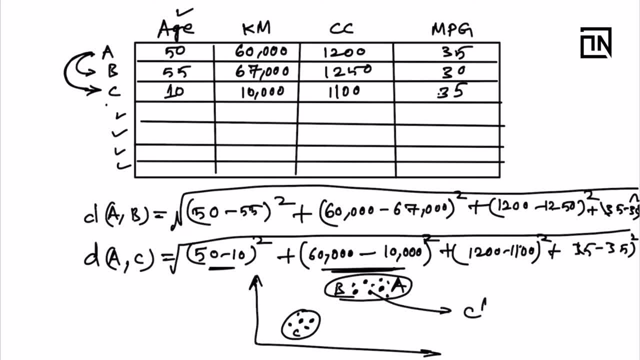 over here. this structure is a cluster or a group, so all the points which you have you have will be somewhere close to it and the point number C will be far away from it. in the data they represent one row and if the row is similar to some other row, 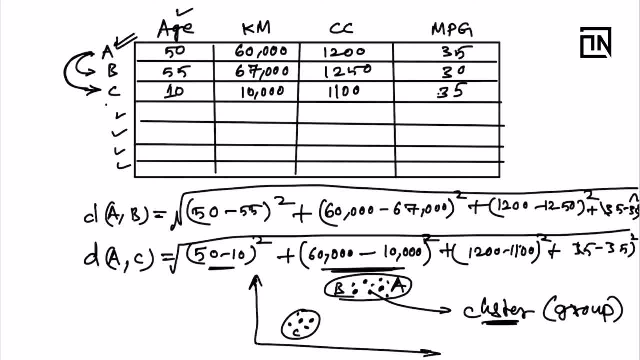 when you plot it, it will appear close to each other because, as the logic says, the distances between them will be very small, because if the values are similar, the difference, the difference between these values, will also come very similar or close to zero, and henceforth the distances 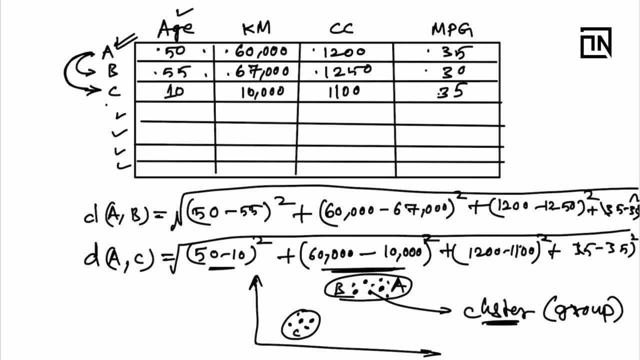 will also become close to zero, so the distances will also be small. so we calculate these distances and then, based on that, we figure out that, okay, this row number a is similar to which particular row, and then, based on that group, okay. so this is the general idea, or the core idea you can say. 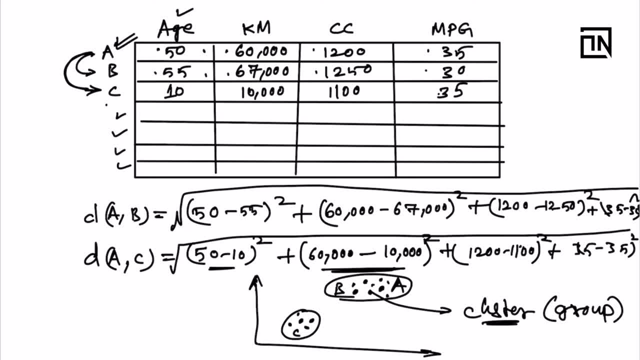 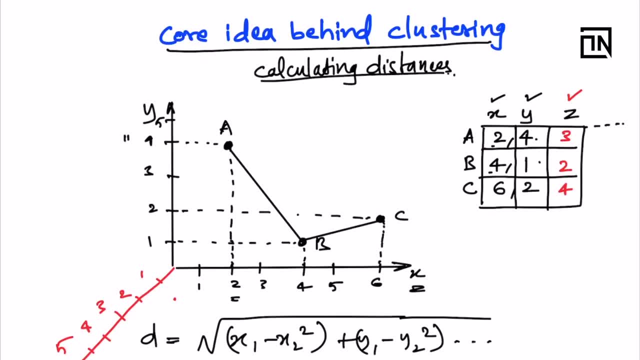 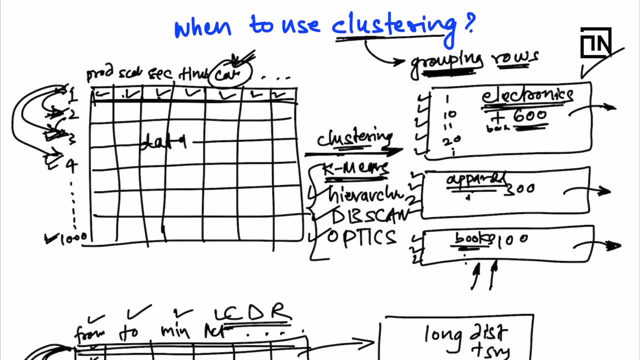 behind all sorts of clustering algorithms. now this distance calculation can be used in multiple ways and people have been really creative with it, and that is why you have other algorithms also in place, like how to how to parallel clustering or db scan or optics. but at the end, at the very core of it, the whole idea is: 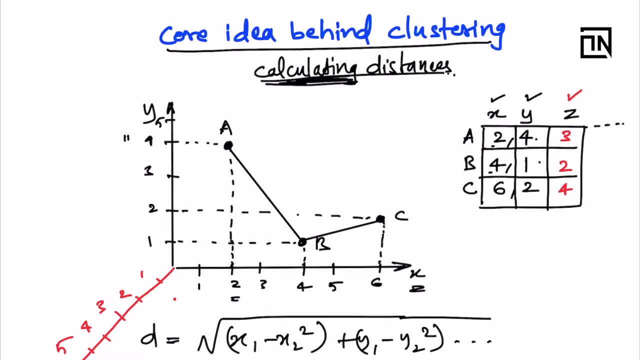 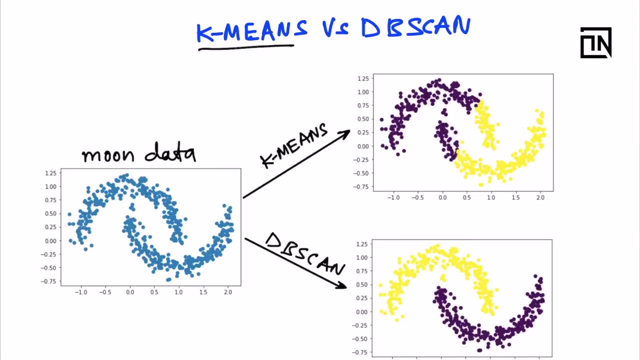 to calculate the distances and then try to bring the groups in some of the other ways. so how do we bring the groups along? that varies from algorithm to algorithm. all right, so now let's understand where k means fail and db scan is able to give you results in that scenario. so 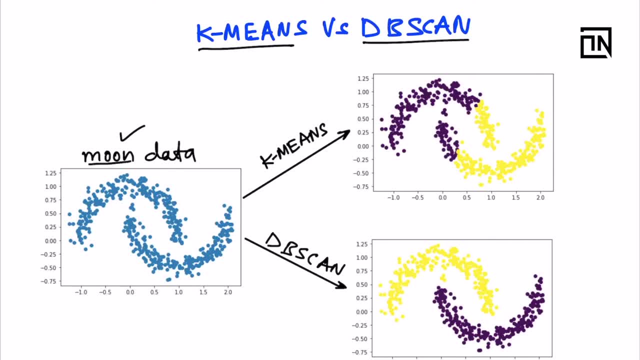 i'm taking the help of the moon data, which is a pretty famous, noisy data set available in python using make moons function, and here you can see it is getting intermixed with each other, so it is coming over here and it is coming over here. so so one particular cluster is kind of merging with another cluster, and this is what 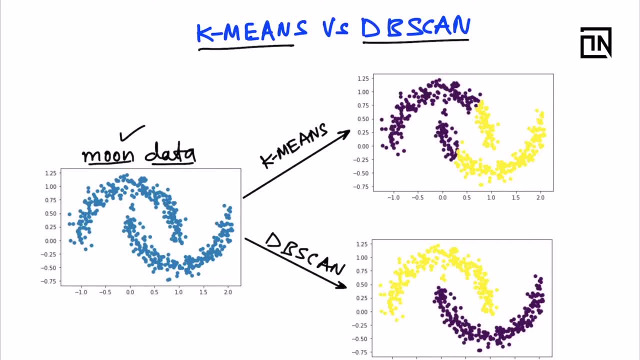 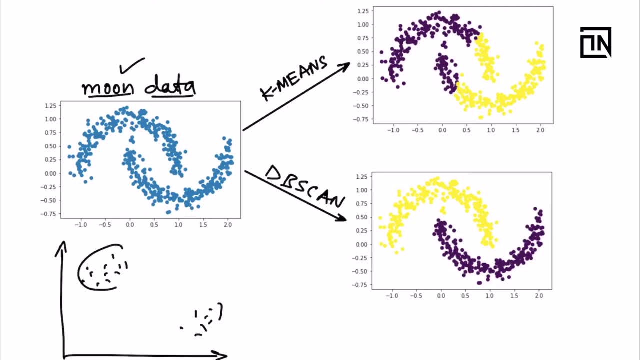 we call noise, so it is not separate. previously we saw that the kind of clusters which we had were grouped in one area and grouped in another area. so we happily created one cluster like this and one cluster like this, so your k means and your hierarchical cluster. uh, hierarchical clustering algorithm will work in this scenario. but if this is the scenario where 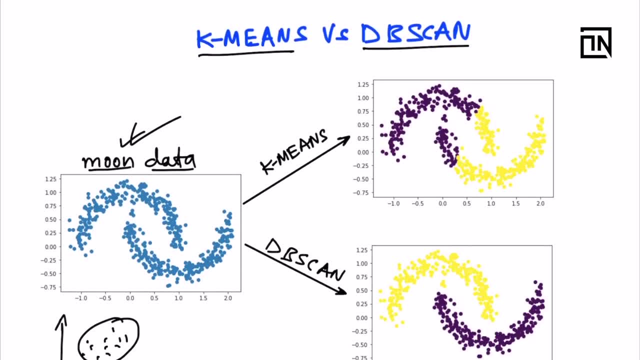 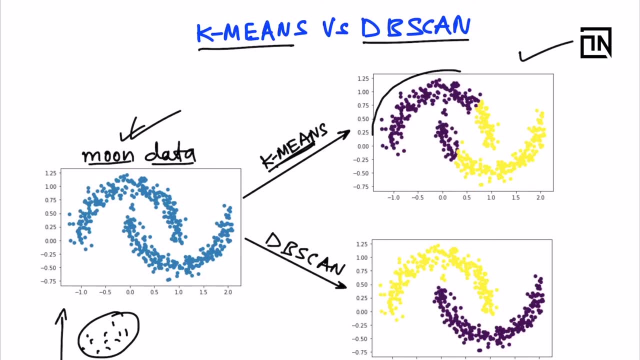 the data is intermixed when there is a noise, then if you try k means or even hierarchical clustering, you will get this kind of result where you will get wrong impression of the cluster. so this is one cluster and this is another cluster, which we can see literally is wrong. the reason behind this is the way k means and hierarchical. 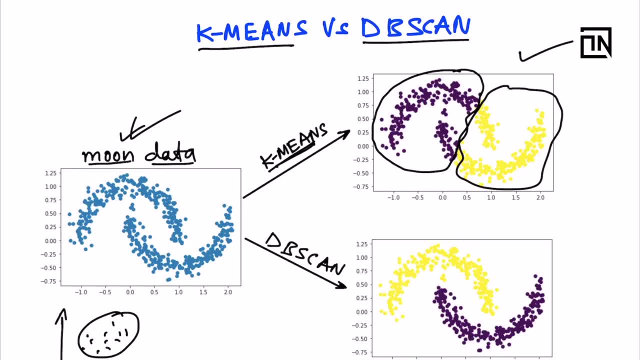 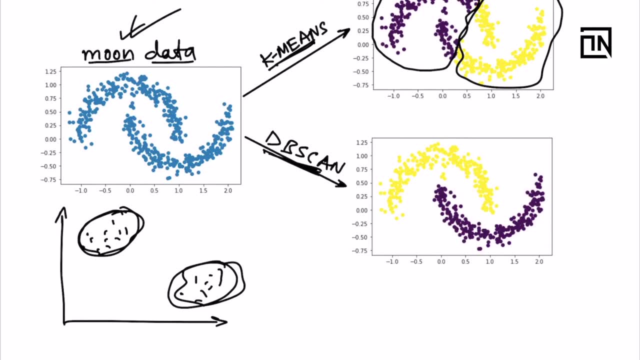 clustering worksгор work. they tend to create spherical clusters. they always try to find out clusters which are spherical in nature. but db scan doesn't work like that. so we will. we will shortly discuss how exactly db scan works, but with db scan you will be able to create meaningful clusters even when. 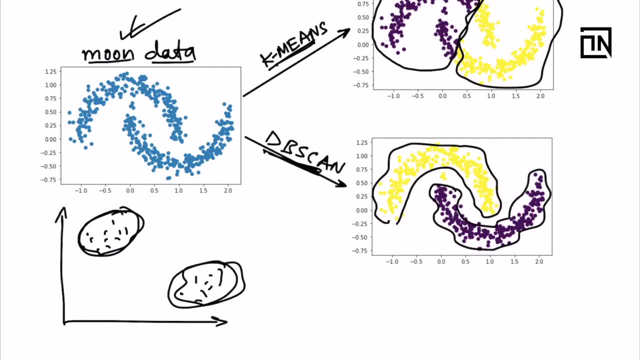 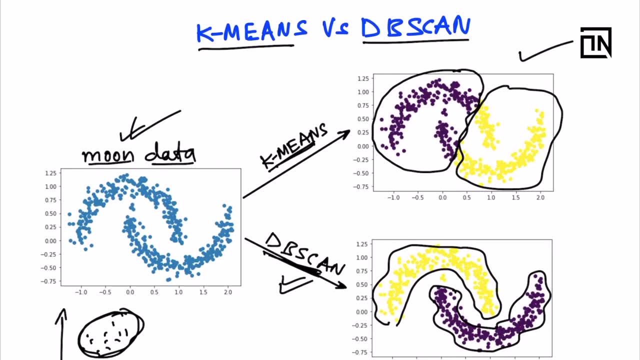 there is noise, even when there are mixtures, you will be able to achieve good clustering results using db scan algorithm. so keep in mind: whenever you have noise in data, whenever you see there is kind of overlapping situations, utilize db scan. it will give you better results as compared to k. 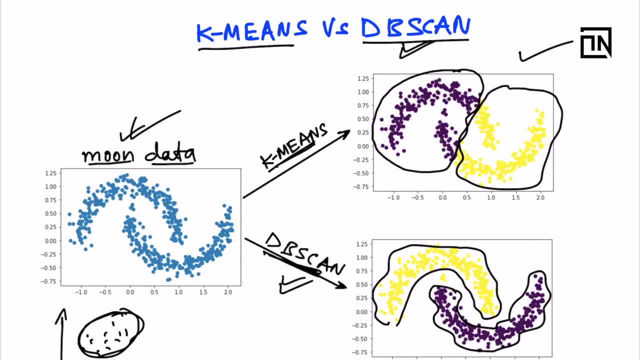 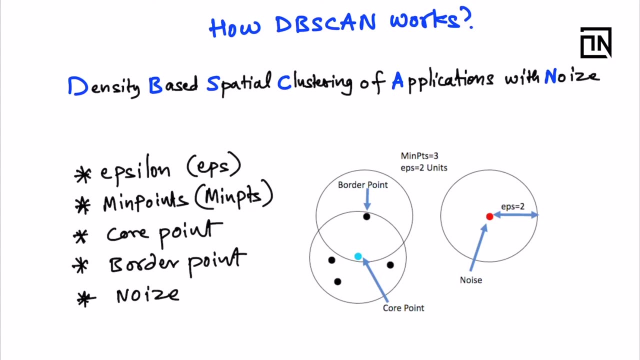 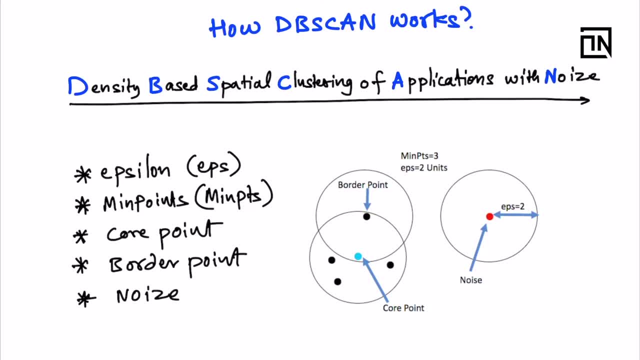 for this long name: density based spatial clustering of applications with noise. you can argue this is one of the most longest algorithm name out there in machine learning world. okay, it's very hard to remember. but yeah, db scan is what we call it in our day-to-day conversations. okay, and if you want, 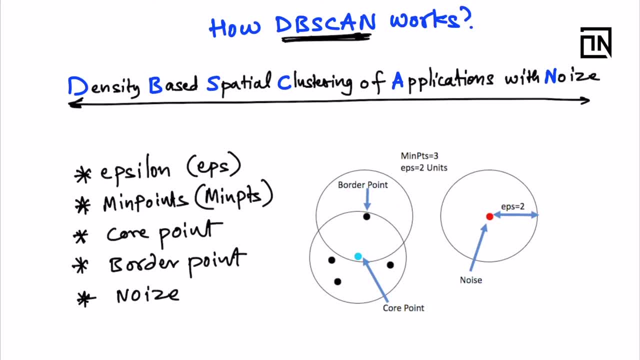 to scare somebody, you can say this whole full form and they will be like: whoa, what is this? what is this algorithm you are talking about? so? so this, as you might have noticed, is density based. so the whole idea of db scan is to find out those groups which are nearer to each other and they are forming. 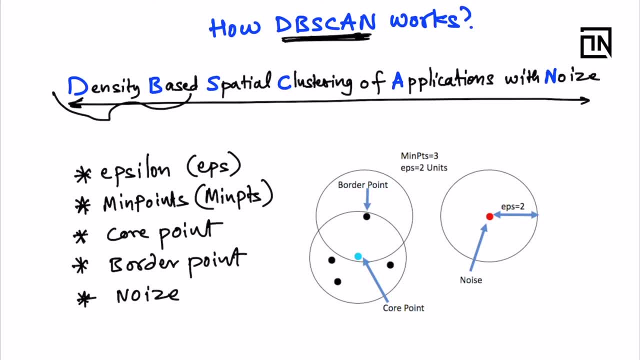 a dense area in the plot. if you do a 2d plot or an n-dimensional plot, it is forming a dense area. so wherever density is high, all those dense points will be clubbed as one cluster, and wherever density is low, that will be clubbed either with the, either with the high density points, or it will be termed as noise, or 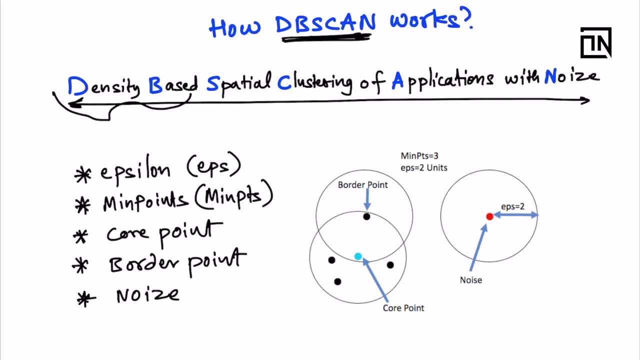 it doesn't belong to any cluster. so there are certain concepts like epsilon, minimum point, score point, border point and noise. these concepts are nothing but the db scan algorithm, exactly okay, so these concepts are internally used. so, first of all, what is epsilon? so this epsilon is nothing but. 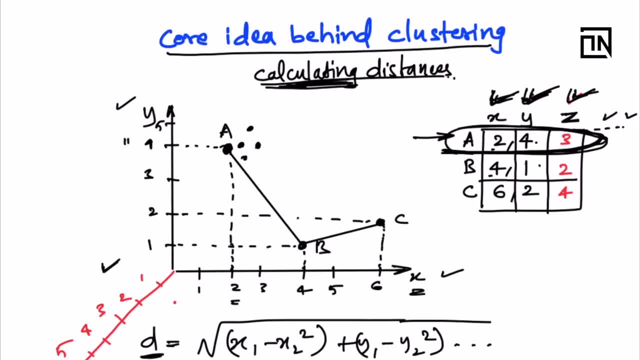 distance between two points. so we have already established this: that you can find out the distance between two points and you can find out the distance between two points, and you can find out the distance between two points and you can find out the distance between two points using euclidean. 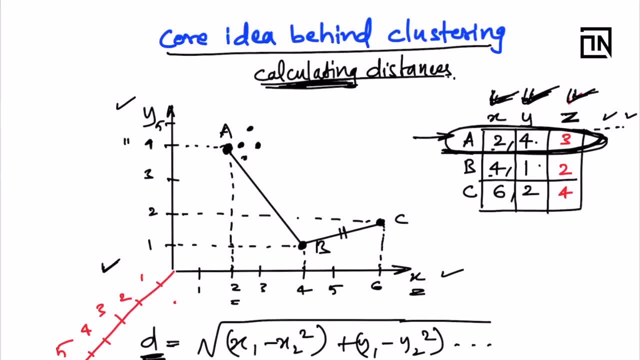 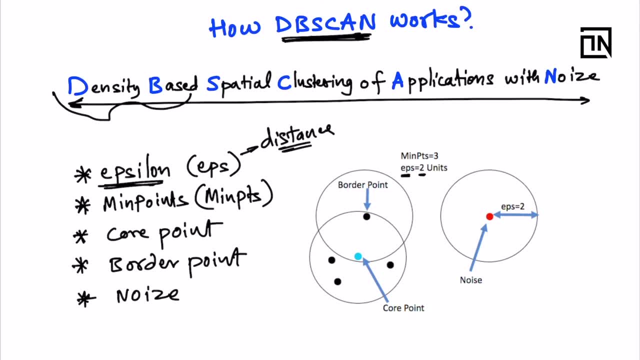 distance using this formula. okay. similarly, you say: i need, uh, epsilon of two units. so two units is nothing but a sample example, for, for distance between two points, like for example over here, this radius which we have drawn and a circle around it is with an epsilon of two or within two units of. 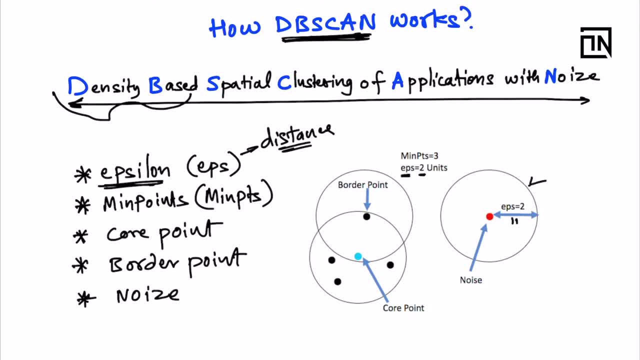 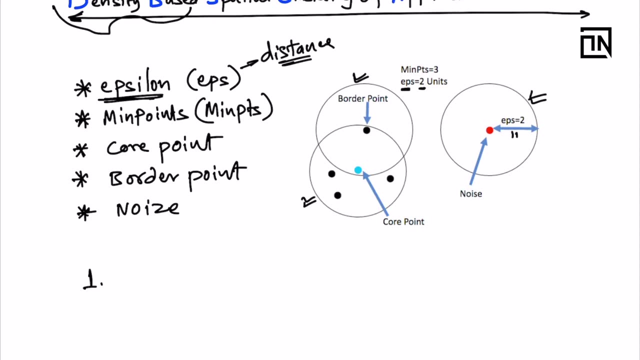 distance, whatever area is covered, i am just marking them using this circle. okay, similarly this circle and similarly this circle. now where I begin this? so I begin this at any random point. so the step number one for db scan algorithm is: choose any random point, begin by any random point. 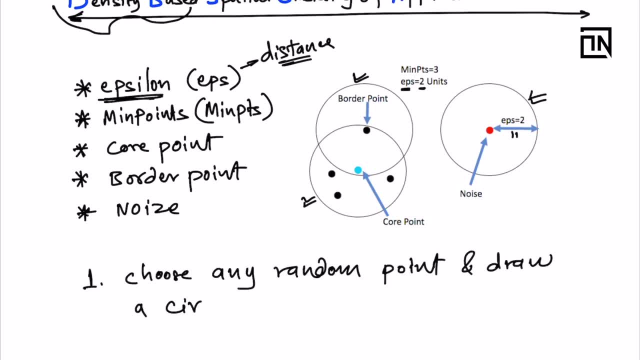 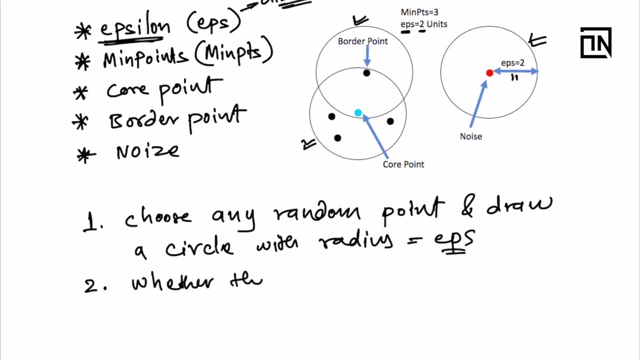 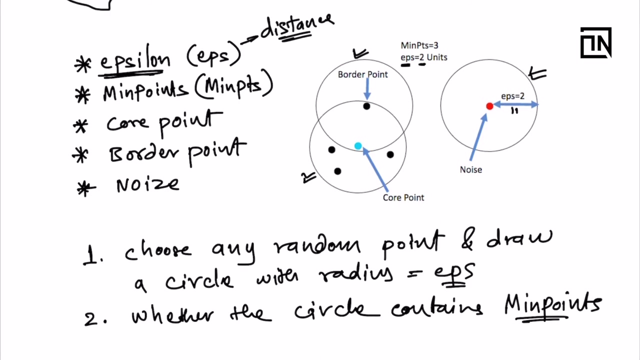 choose any random point and draw a circle with radius equal to the epsilon. so for any random point, I will draw this circle and then, in the next step, I will see whether the circle contains minimum number of points, which I want. so I can define this minimum number of points and 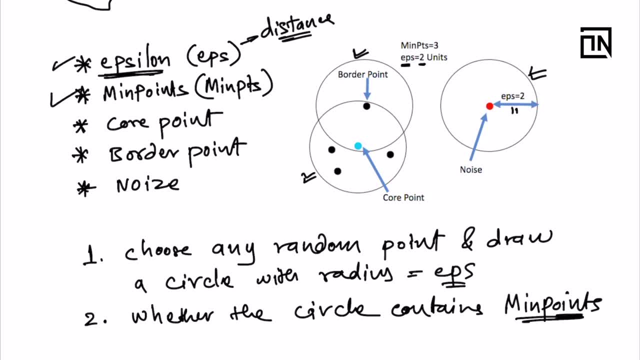 epsilon and minimum number of points. these two are the hyper parameters of db scan which we tune when we fit the algorithm onto a given data. now, if I have specified that I need three points, so within this circle which I have drawn, this circle, I will draw this circle and then in the next step I will see. 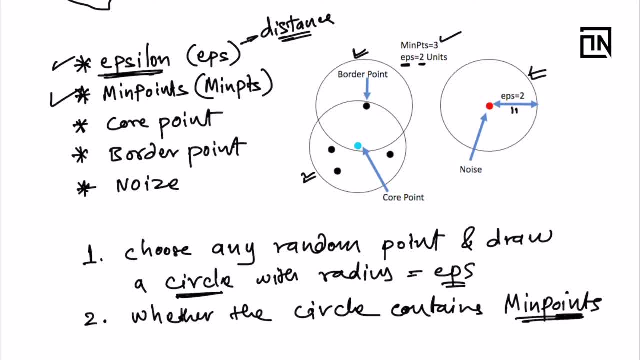 I have drawn, I will try to see whether there are three points or not. if yes, I will call that point a core point. if there are minimum number of points, minimum number of points, let's say, let's say this circle, consider this circle. so the blue point is a core point, because when you created a circle, 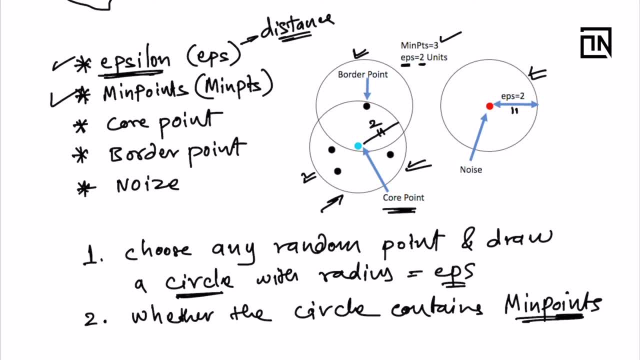 with epsilon is equal to two. you found three points inside it, or in fact in fact four points: one point, two point, three point and four points. so four points inside it. so it is greater than minimum number of points required. so if any point satisfies this condition, then you say: 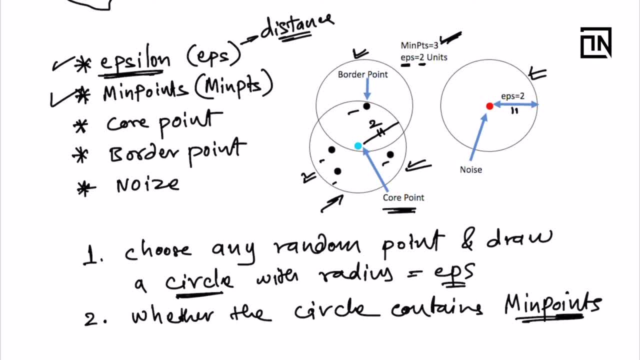 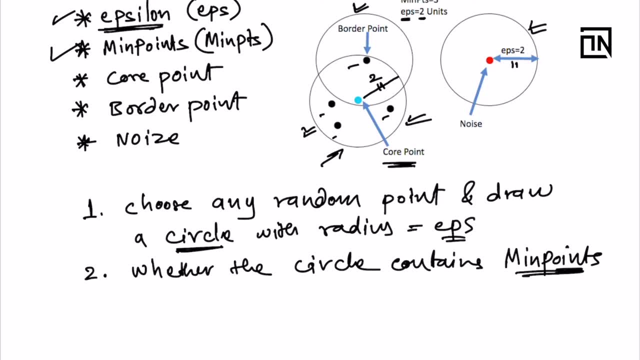 this particular point is a core point, okay, and then you do this process for every other point which is not being attended. so so you begin from here, and then you will say that now this point is covered, this point is covered, this point is covered, so let me proceed with other points. 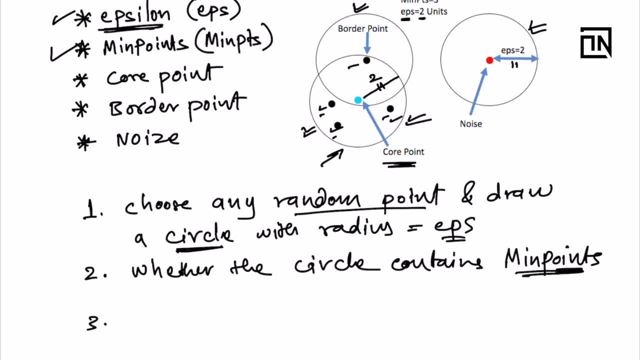 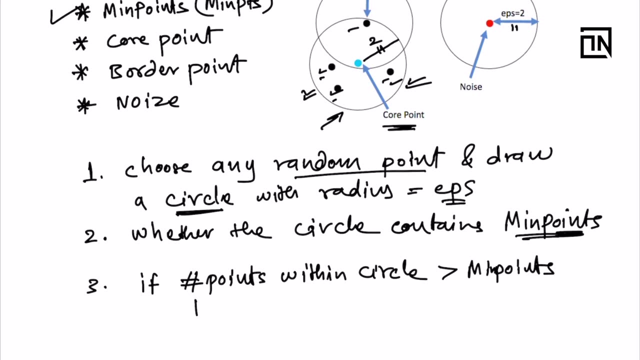 so you start with any random point and then we repeat the step 1,, 2 and 3.. So what is the third step? Tagging. So if the number of points within circle is greater than min points, I will tag that particular scenario as a core point and I will group. 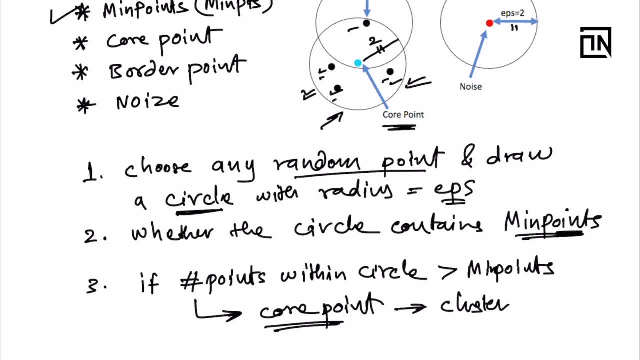 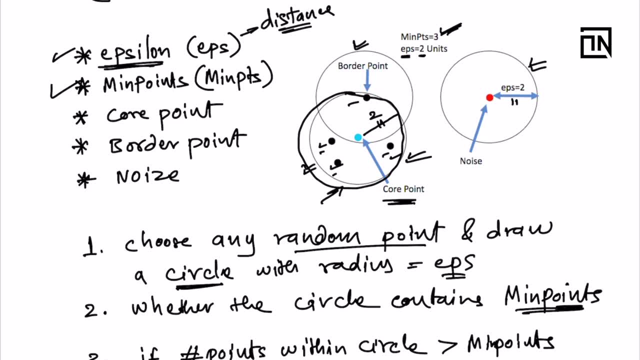 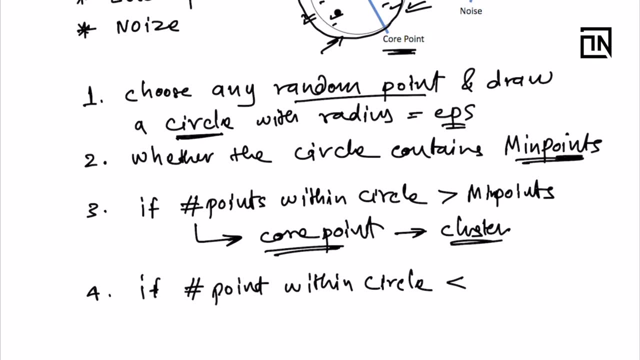 all these points as one cluster, I will say: you all are one cluster. So for me now, this circle is telling me that this whole thing is a cluster in itselfOkay, If the number of points within the circle is less than here, let me add the class equal to less than main. 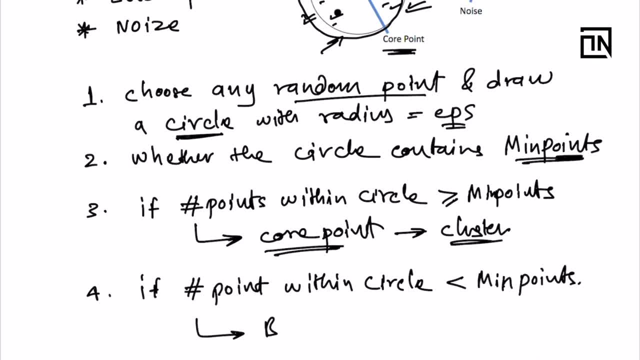 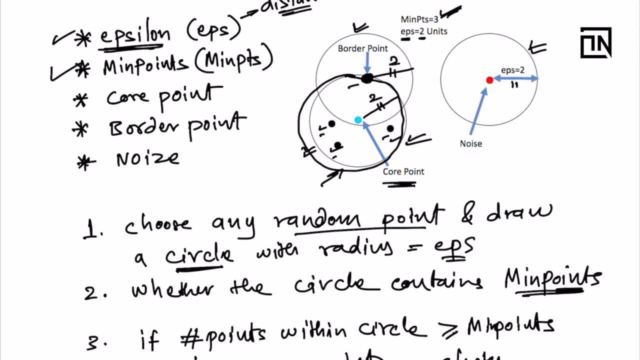 points, then we say this is a border point. Okay, So this is a border point. This particular point is a border point because when you created a circle using two epsilon, there is only one point which came in its circle, which is less than the circle. 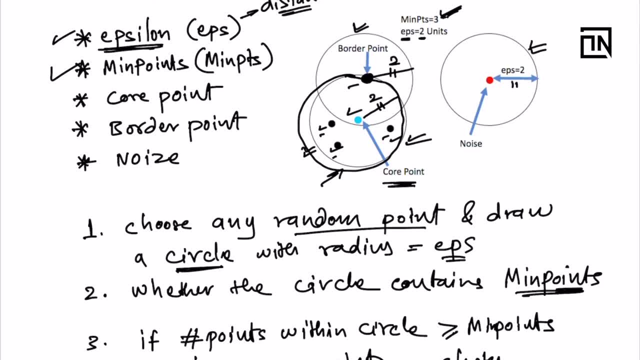 minimum required points of three values which i have specified. this is something you can change in every data set. you can start by min points equal to 2, 3, 4, 5, 6, and you can raise the epsilon value also like 1, 1.2, 1.3, 1.4, so on and so forth. so whichever combination gives you the best results, 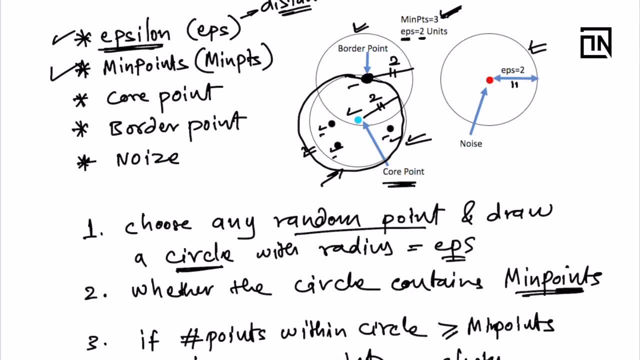 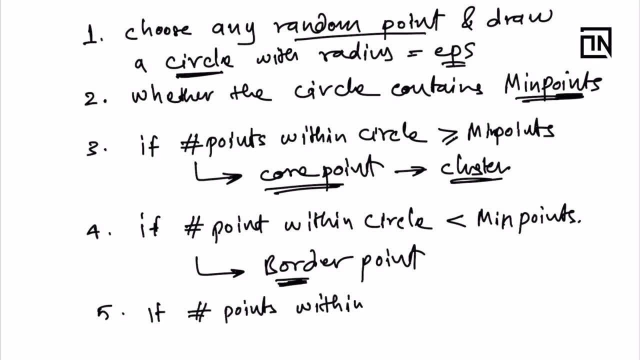 you will choose those two. okay, and how do we know it is the best result? we use the silhout score, so this is categorized as border point, and if the number of points within circle is equal to 0 means there are no other points, then we say this particular point is a noise, which is the scenario. 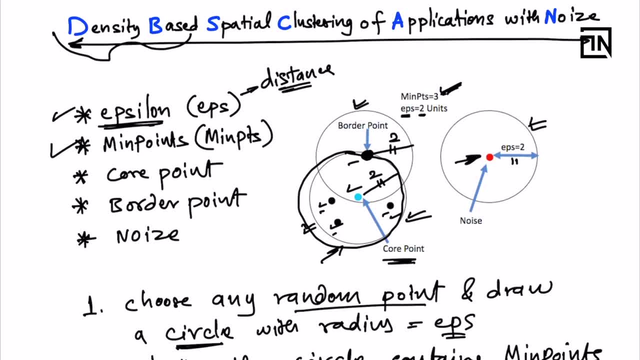 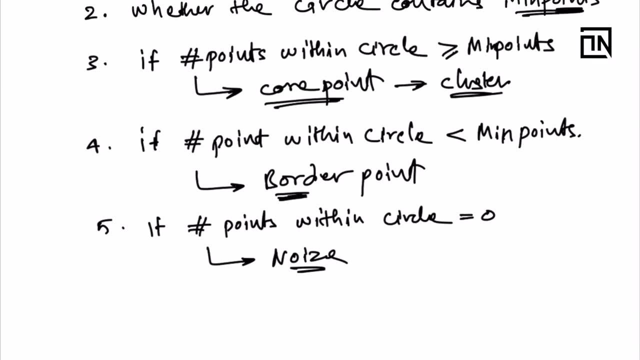 this is a noise point. why? because within its circle of epsilon 2 there are no other points. there should have been some point, at least one, two, three, any number of points, but there are no points. so very simple: three tagging cases happen for every point out there in the data. so in your, in your data set there might be multiple such. 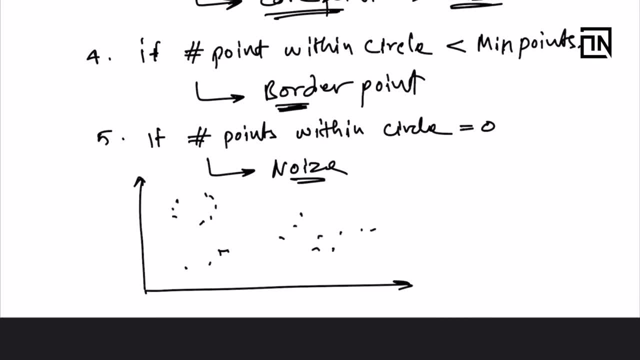 points like. some points are here, some points are here, some points are here. so what you'll do? you'll begin by this point. you'll draw a circle, you draw a circle, you draw a circle, you keep on drawing these circles for each points and you keep on tagging them, whether they contain. 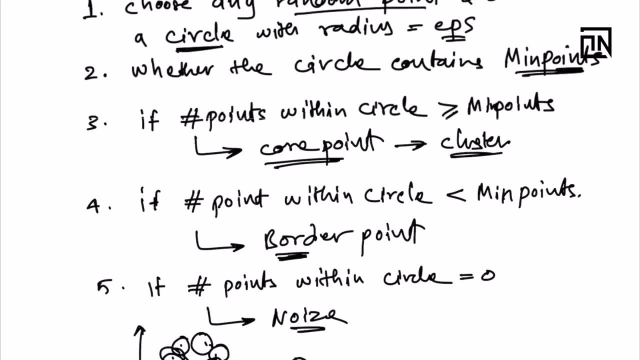 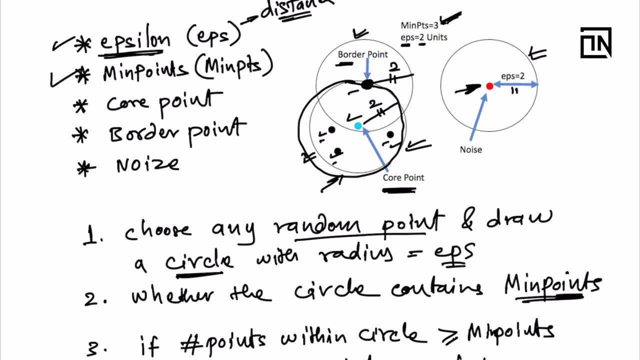 the minimum number of points or whether they are far away from most of the points. so this is done for every point, and then each point is either denoted as core point or denoted as border point or as a noise. so noise is something which is not belonging to any group or any cluster. and core: 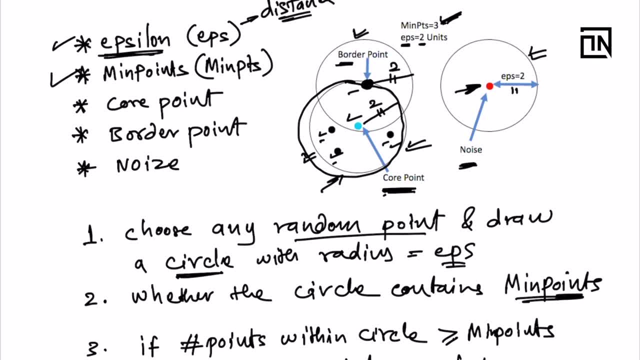 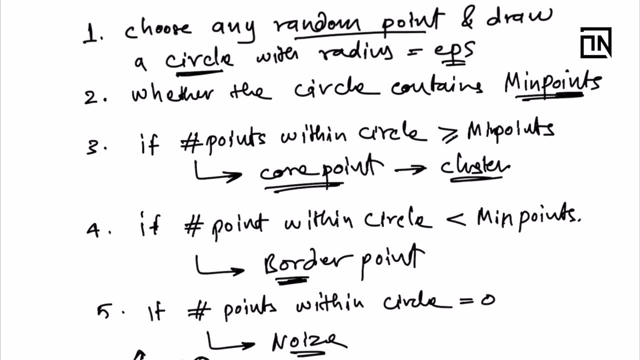 point is a cluster in itself, it is a mini cluster in itself. this particular point is a mini cluster in itself. so these one, two, three, four, five, these points are nothing but one cluster. so next, what we try to do is we have tagged all these points and then we say that whatever. 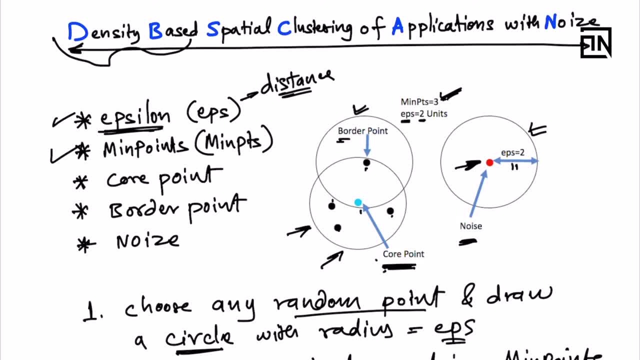 is whatever core point is there which is touching any border point, the circle of any border point, those two circles now will merge together like this: these two will now belong to one particular cluster. similarly, if there was one more point and and the circle of that point was touching, 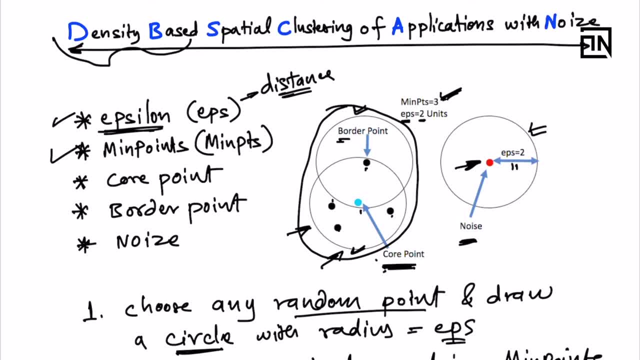 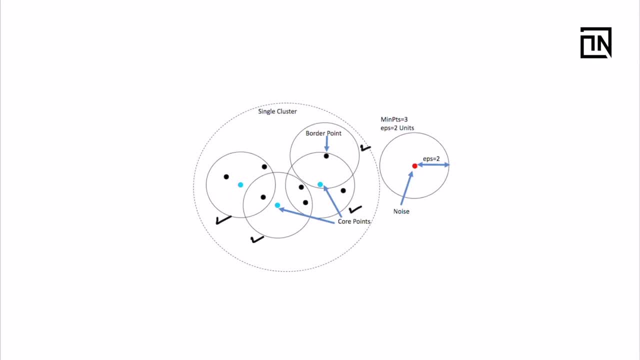 the circle of this core point, then they also will be merged together. so a clear example would be like this: look at these circles, this circle, this circle, this and this. so all these circles are kind of similar. so all all of these points belong to now one single cluster. there might be similar kind of 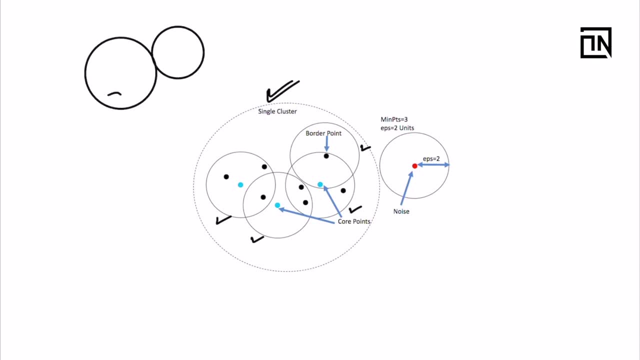 clusters over here as well, like there will be points which are touching each other over here, like this: now these, these points which were there, they are not able to touch these points, so this whole thing becomes one different cluster and this whole thing becomes one cluster. so now we have a particular point which is not coming into contact or which is not near to any. 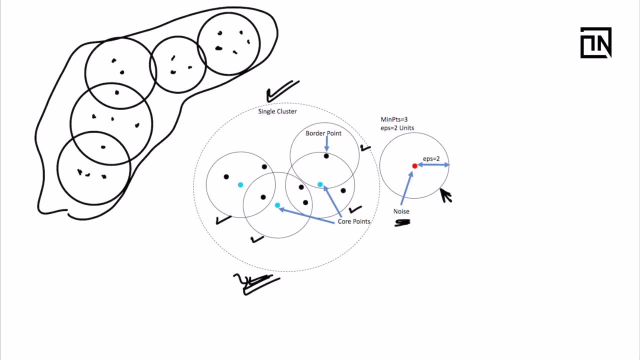 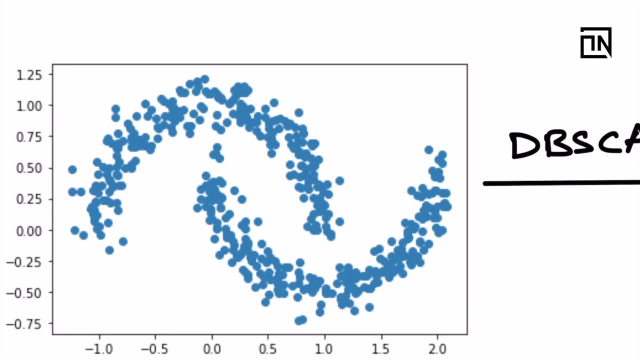 other point. this becomes noise, so this actually starts a chain reaction. what it does is it says: okay, i'm starting from here. so this starts to draw its own circle like this, so it touches the circle of this point. this touches the circle of this point, this point. 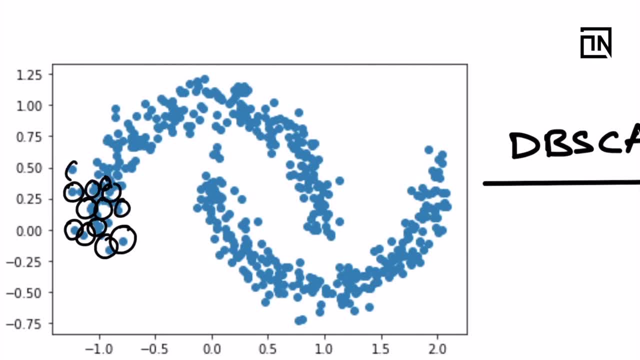 so all of them touch the circle of other points. somehow, some of them will be core points, some of them touch the circle of other points and this process continues and this chain reaction happens. and all these points which are there, which are densely close to each other, which are 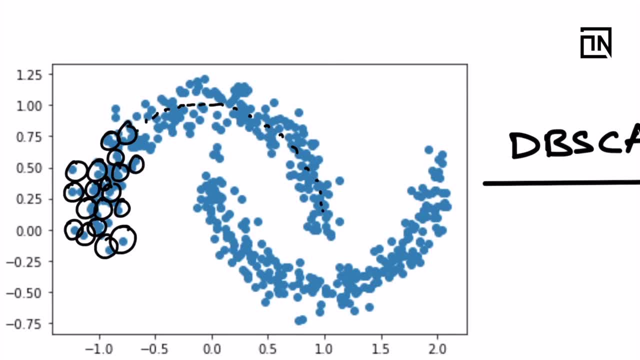 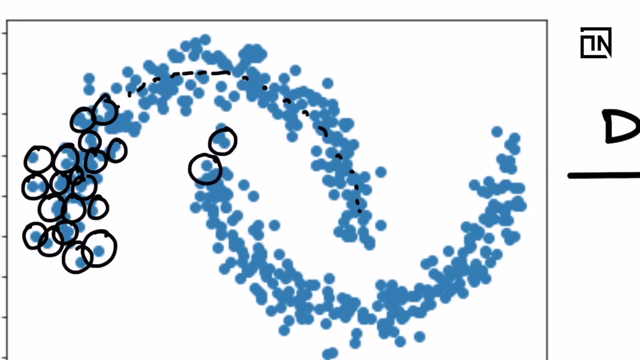 which are kind of near to each other and they are forming a higher density. in this area now, where the density is low, like in this area, in this region, where the circle is not able to touch each other, they are, they're kind of falling by a little margin, so they will start their chain reaction. 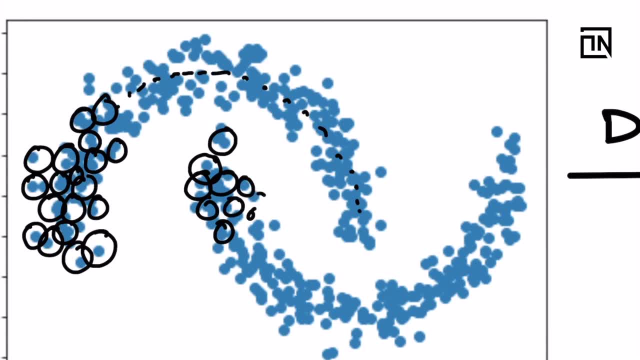 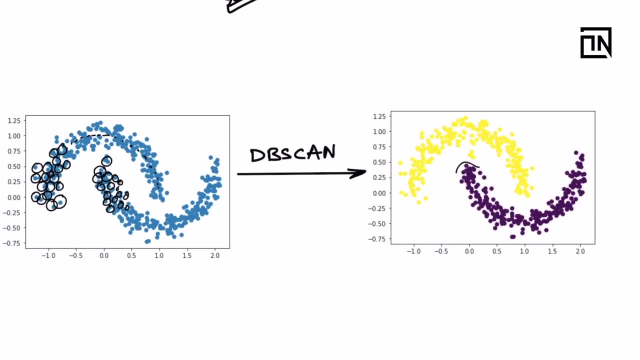 on the other side and their clustering will be done or their grouping will be done. so this is how db scan is able to achieve these kind of boundaries which you see over here, based on this chain reaction which has happened now, if you change the epsilon, if you change the, 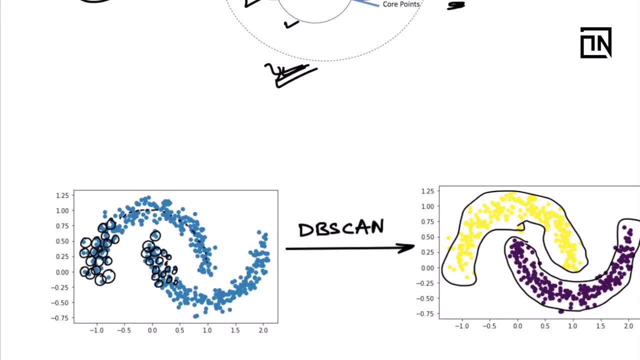 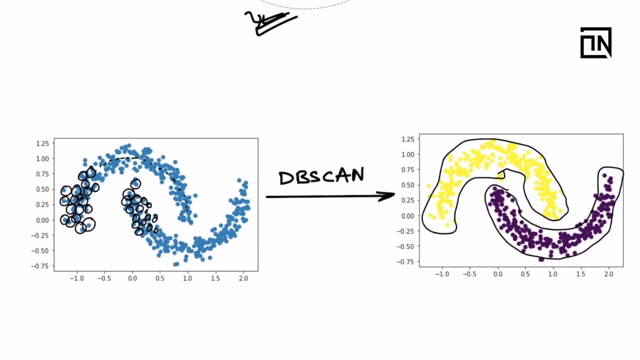 value of epsilon. this will greatly affect the way it will create the clusters. now let's say, if you choose, epsilon is equal to five. now, five is a bigger circle, so every point will create big, big circles. now over here, so most of the points will be accompanied. 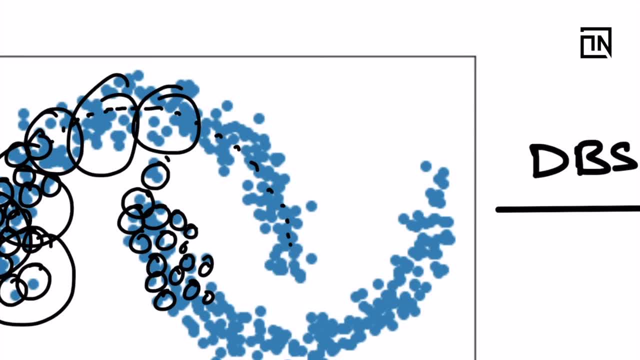 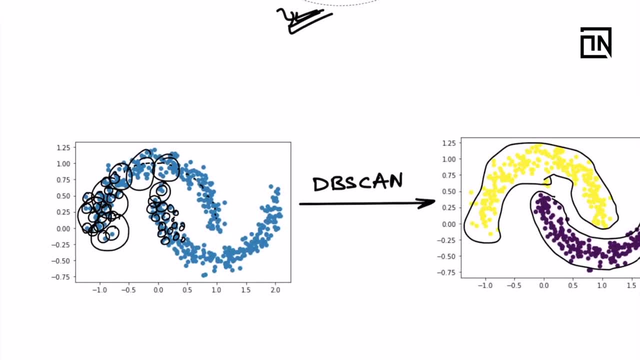 now here this circle which was not able to touch the other circle, now this will also touch it. so the whole thing will be one single cluster. so the epsilon is really critical parameter in db scan. if you choose a really large epsilon, then the whole data point or the whole data set will become. 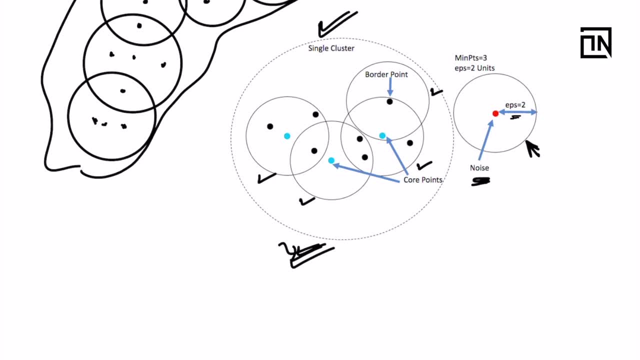 just one single cluster. on the other hand, if you choose this epsilon very small, then these points will not be able to touch each other and this is how you can create a big, big circle over here. so you can create a big, big circle and you will get so many clusters. so the epsilon value is a. 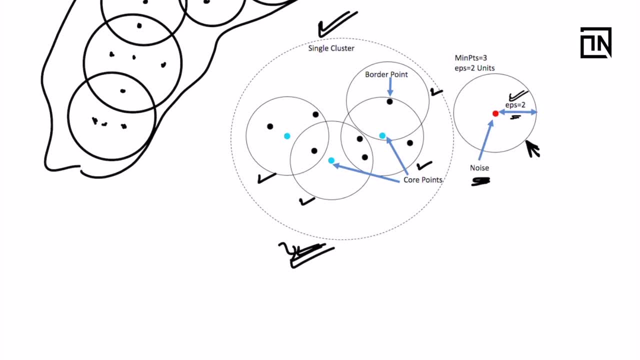 very important hyper parameter in db scan. it determines what kind of clusters, or how many clusters, you will get in the given data. okay, similarly, the minimum number of points, because this is the criteria which you define, to call any point as core point. if a point is a core point, so 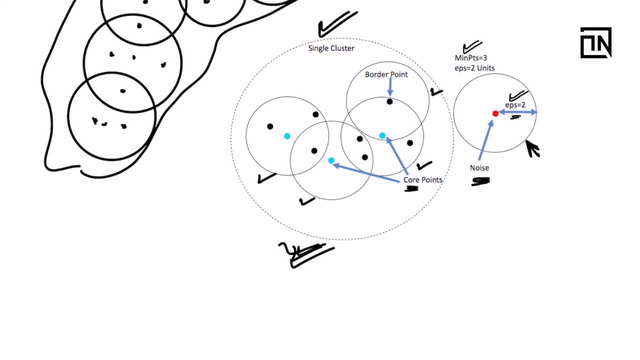 by default it is a cluster in itself and the moment it starts touching the cluster boundaries of other core points, all those are included in one single cluster, so on and so forth. So minimum number of points and the epsilon value, these two actually drive the whole dbScan algorithm. 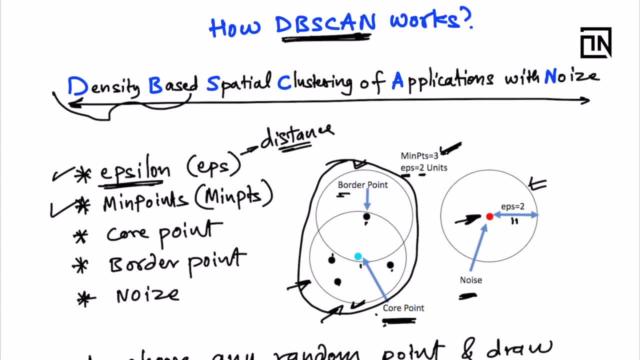 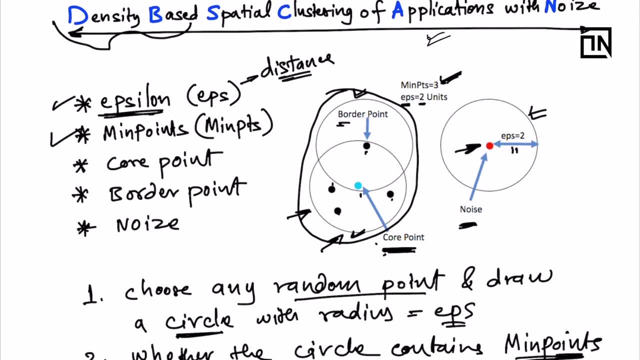 Now you see it is so simple concept. only the name was kind of complex, but the whole procedure which we have inside dbScan is pretty, pretty simple and this is why, on large data sets also, it will work very fast and will be able to give you meaningful clusters. 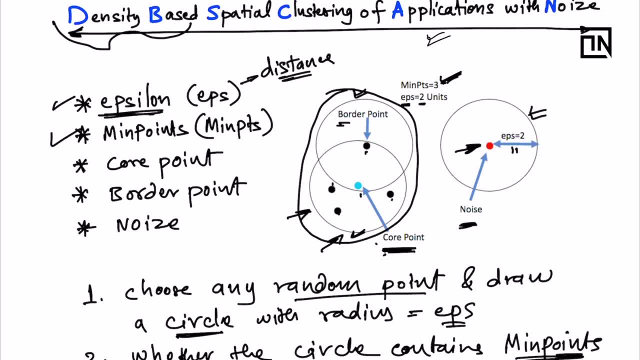 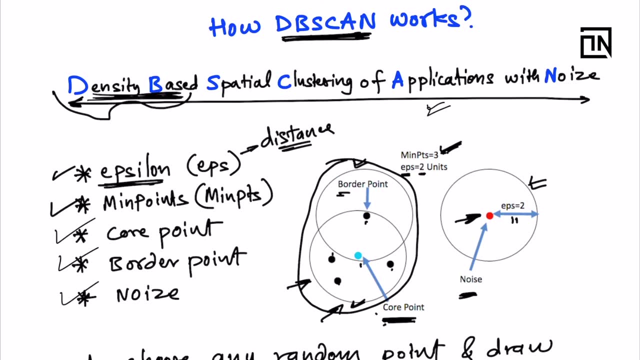 especially if the data has noise. okay. So these concepts which we just understood, the core point, the border point and noise, these concepts only- are driving the dbScan algorithm, which is density based. So wherever higher density will be there, the dbScan algorithm will group those points. 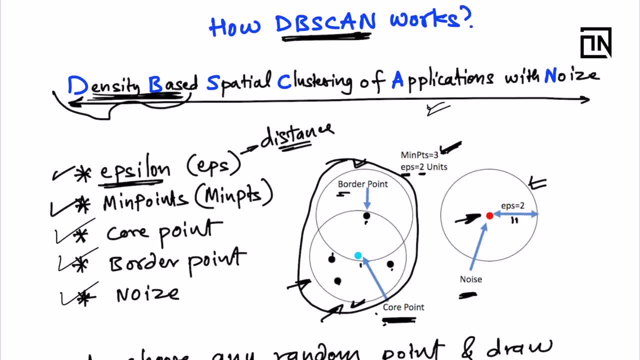 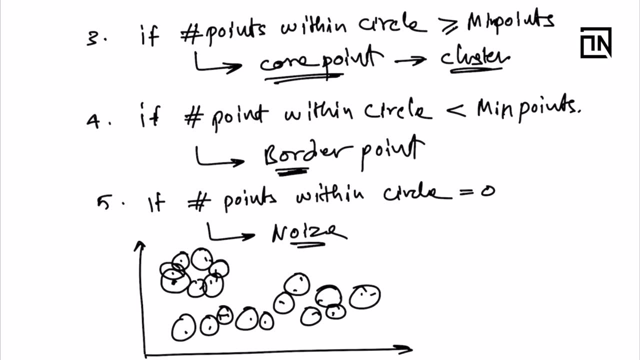 and wherever the density is smaller. if the density is so low that the points are alone, then it will tag it as noise, it will not belong to any group and the other other lumps will be formed in the data. So one, so over here the traditional example of clustering. 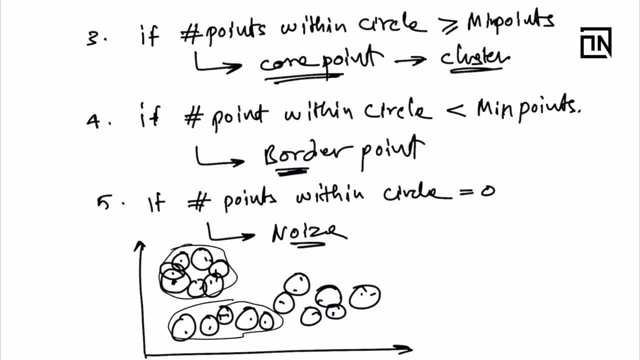 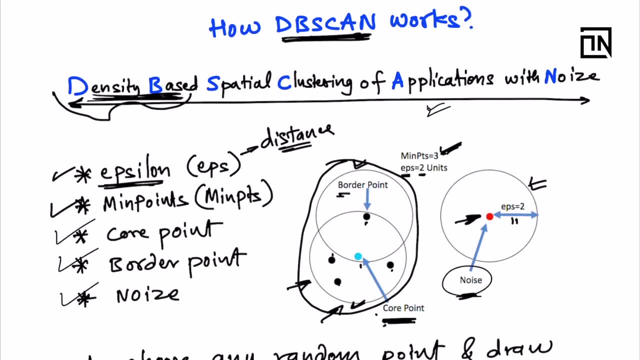 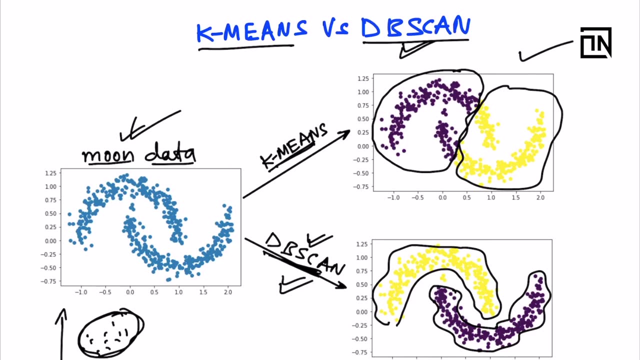 like, one whole cluster will be formed here, one will be formed over here, one will be formed over here, and maybe one or two points will be termed as noise. okay, So dbScan algorithm has an advantage over k-means and hierarchical that it will be able to give you clusters. 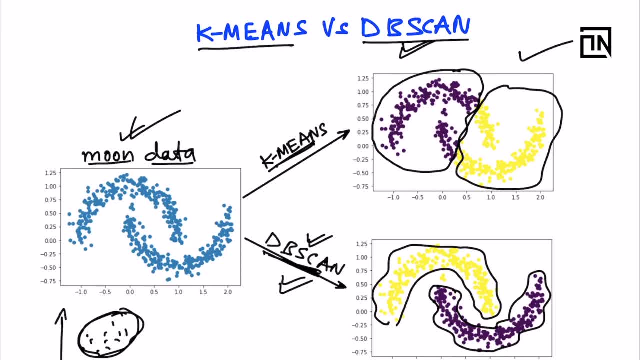 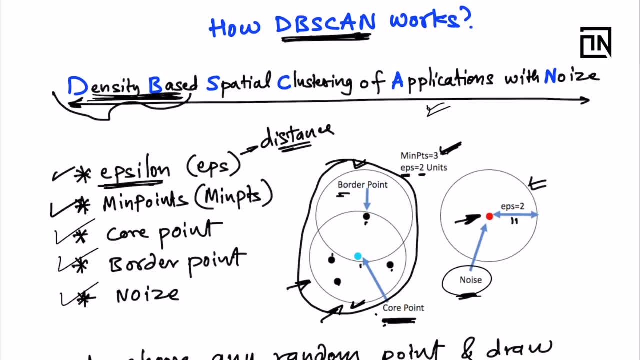 on those data sets which are having noise or which are intermixed with each other also okay, And in the interview typically the questions revolve around what will happen if I change the values of EPS and choose a very small value, So you will get many more clusters. 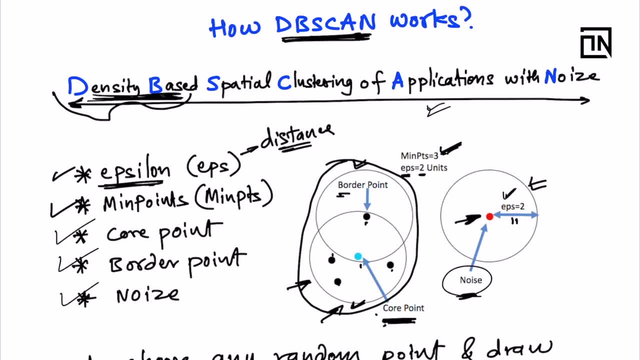 What will happen if I choose the EPS as high? So you will get only one cluster and it is very sensitive. So that is why, when we tune this parameter, we increase the values by a very small amount, Let's say 1, so 1 and 1.01,, 1.02, like this: 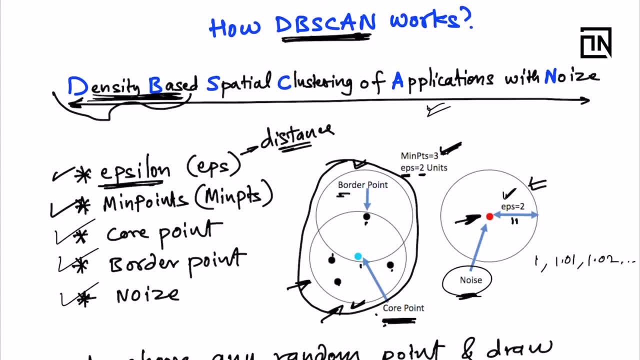 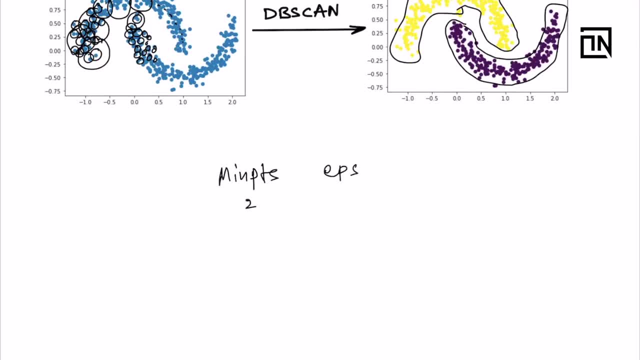 We increase by very small amounts And then for each combination, let's say we create a table, mean points, mean points equal to 2 and epsilon is equal to, let's say, 0.1, mean point equal to 2, epsilon 0.2, mean point equal to 3, epsilon 0.1,.